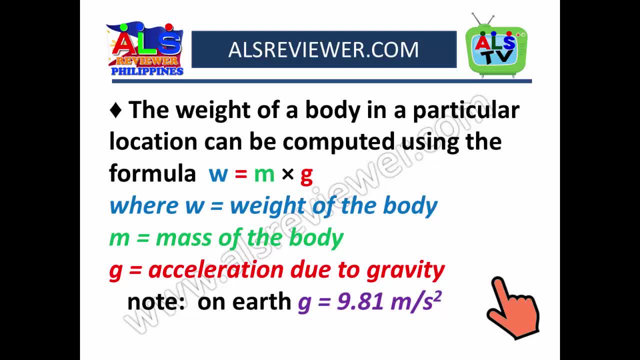 Because mass is the composition or elements that makes up a body. So, for example, how much is the composition of that body, our body, for example? how many elements are formed here? Meanwhile, weight- weight of the body is affected by the gravity. 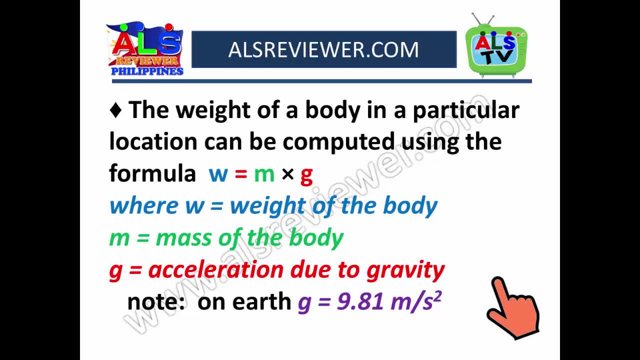 So what we're talking about here is the force exerted by the Earth towards any object. This means that the closer to the magnet, for example the literal magnet, the closer the object or the metal to the magnet, the stronger the force. 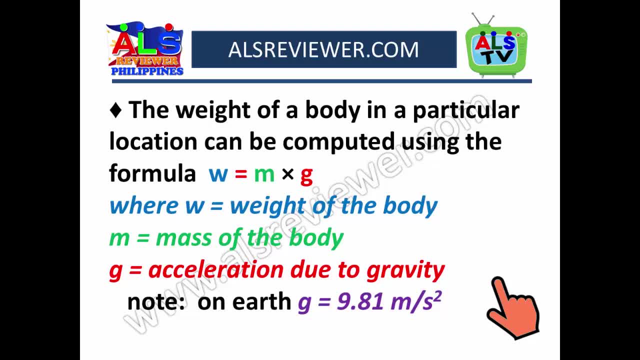 Meanwhile, if you move it further away, while it's further away the magnetic field will weaken, And if it's further away, the magnet will weaken in that object. So that's the effect of the weight of the body, The so-called W and the mass. 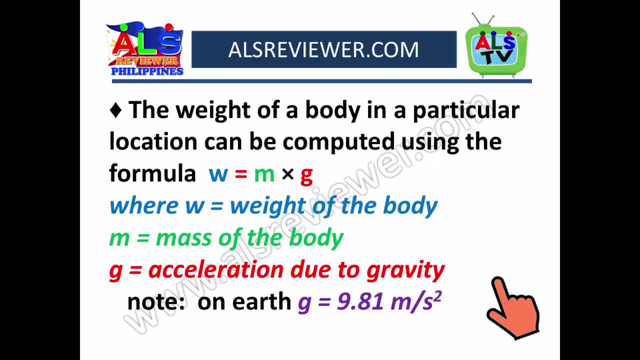 The mass doesn't change. Okay, Let's see. What we're saying here is that on Earth, g is equal to 9.81 meters per second squared. Okay, So this is the constant wave of gravity here in the world. 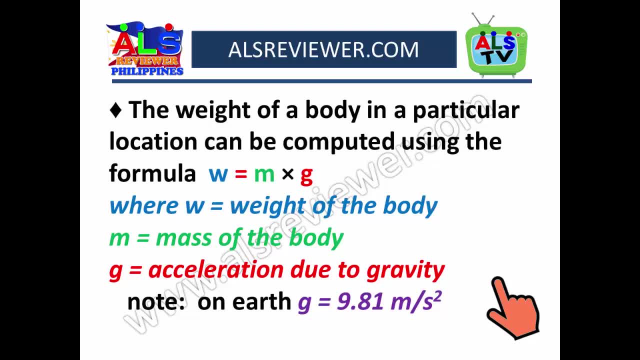 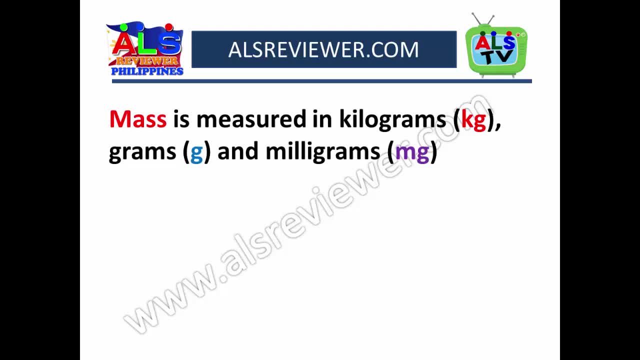 Okay, We'll understand that as we go along. Okay, The mass is measured in kilograms. The measurements used here are grams, kilograms, milligrams. Okay, Weight is measured in tons, Pounds, ounces and kilogram meters per second squared. 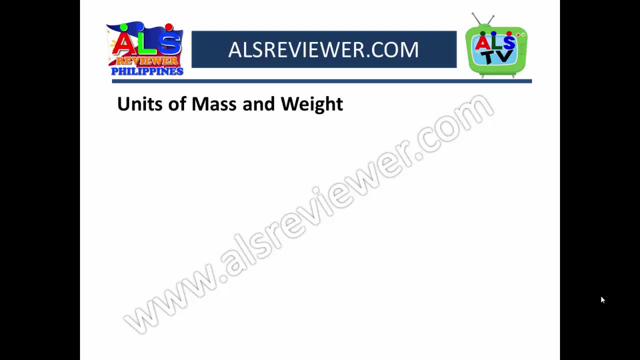 Here are the units of mass and weight. For example, 1 kilogram is equal to 1,000 grams. When we count in kilograms, the gram is 1,000 grams. That's 1,000 grams. Okay, Equal to 1 kilogram. 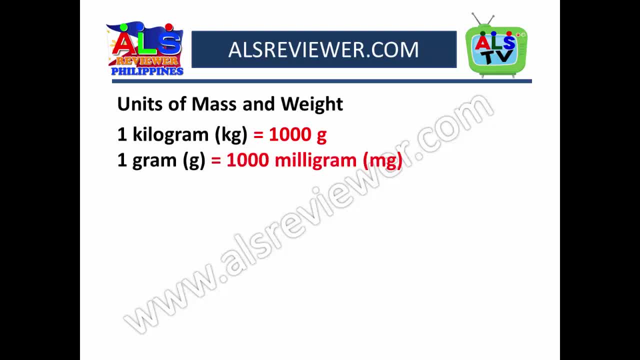 Okay, The 1 gram is 1,000 milligrams. Okay, This is a smaller number. The 1 ton is 2,000 pounds. The 1 pound is equal to 16 ounces. The 1 kilogram is 2.2 pounds. 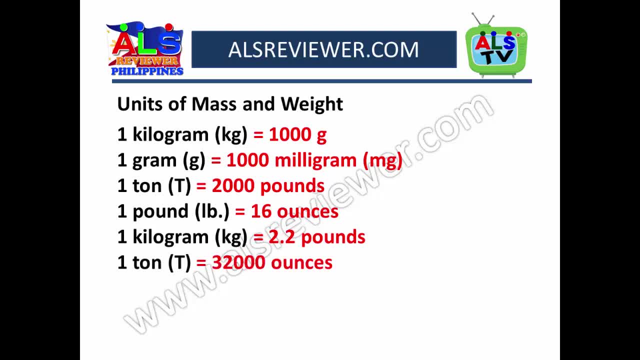 And the 1 ton is equal to 32,000 ounces And the 1 pound is 4.45 kilogram meters squared. Okay, So these are the units of mass and weight. So if there are problems that you need to study and you need a conversion, 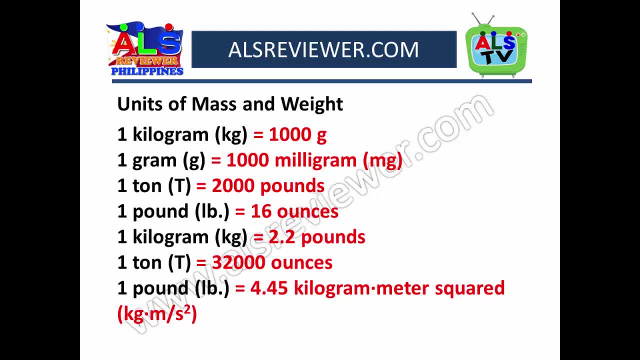 Okay, When do we need a conversion? We need a conversion When the unit used in the problem is different from what the problem requires. Problem or the word problem. Okay, We will understand this later as we go along. Okay, The 1 ton is 907.2 kilograms. 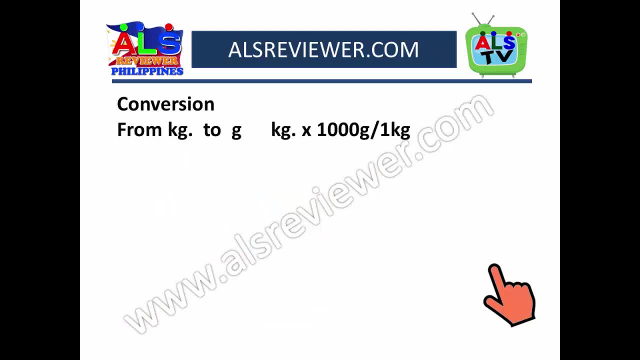 Okay, Let's go to conversion. When we convert from kilograms to grams, Ibig sabihin yung kilogram kilo. a thousand gram, Ibig sabihin yung malaking kilo. titignan natin kung ilang guhit. 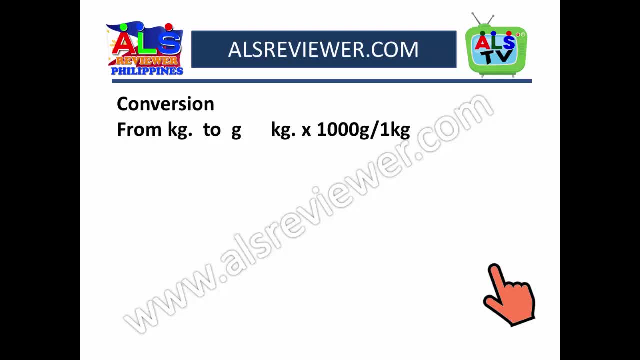 Talimbawa. So dito kilogram A kilogram is equal to a thousand grams, So ibig sabihin yung 1 kilogram dito binubuo ng 1,000 gramo. So paano ang pag-convert natin? 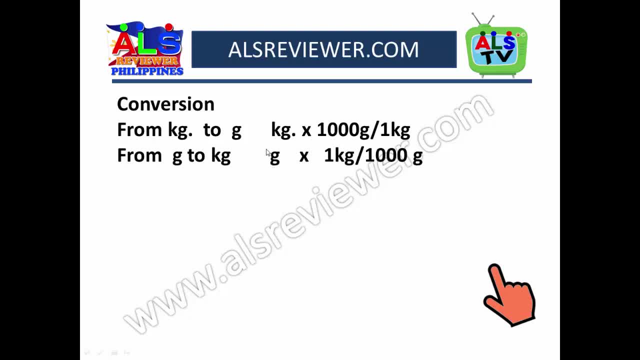 From gram to kilogram, naman Mas maliliit. itatranslate mo ngayon sa kilogram. Okay, So ang 1 kilogram is equal to a thousand gram Namaya, titignan natin dito Example. 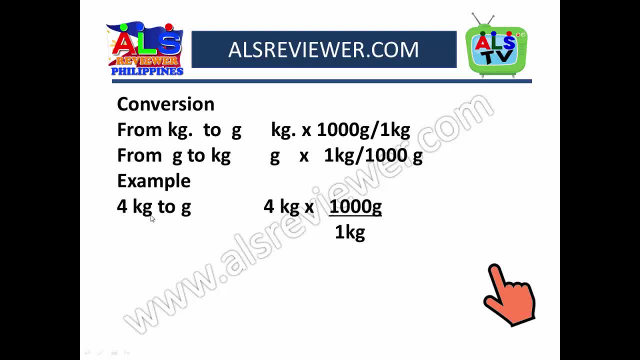 Okay, Talimbawa Yung 4 na kilograms, 4 kilograms. i-reduce natin ito or i-convert natin ito sa grams. Okay, So nalaman natin: Ang 1 kilogram is 1,000 grams. 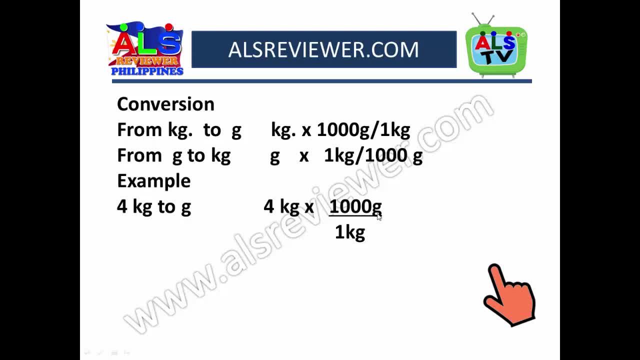 So ang gagawin lang natin 4 kilograms times 1,000 grams. Pero dito ginamit natin kasi ang ratio in proportion para yung units. Yung units nito ay pwedeng i-cancel. 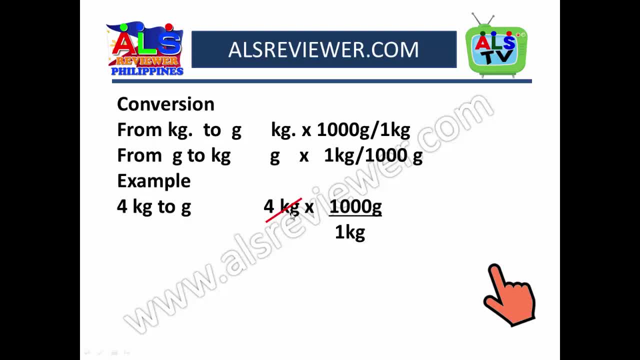 Mamaya, papakita natin. Okay Ayan. So kilogram dito, Kilogram dito, dahil ito ay nasa numerator At ang denominator nito is always 1.. So numerator and denominator cancels out. 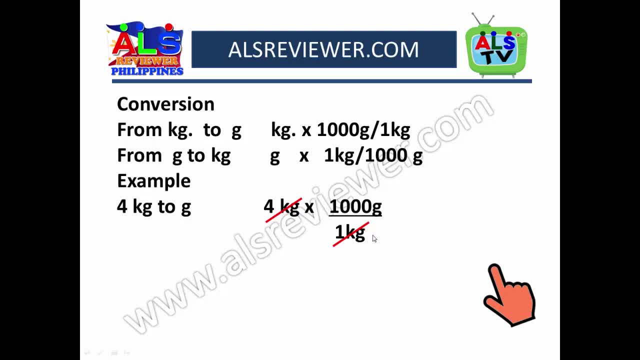 Kaya yung kilogram doon naalis na. Okay, So ang natitira na lang 4 times 1,000.. Ang unit nito is grams, So ibig sabihin na ang sagot ay 4,000 grams. 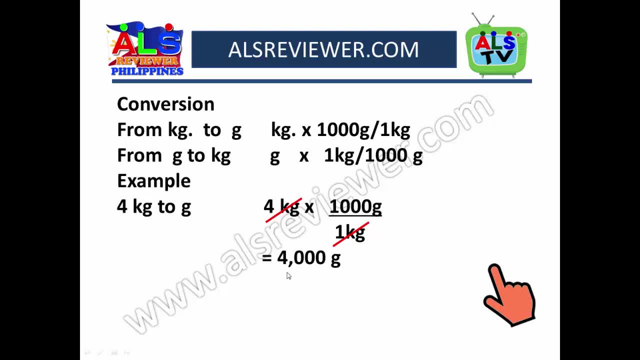 4 kilograms equals 4,000 grams. Okay, Ngayon, Pag sa baligtarin naman natin Yung 4,000 grams, tatanungin natin ilang kilograms ba ang 4,000 grams So mangyayari nito. from smaller unit i-coconvert natin ito sa mas malaking unit. 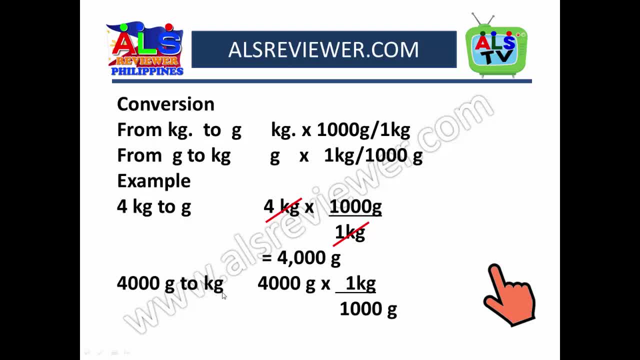 Okay. So grams is a smaller unit, Kilogram is a bigger unit. Tingnan natin 4,000 grams. Icoconvert natin ito ng kilogram. Paano ang gagawin natin? It's just like multiplying. 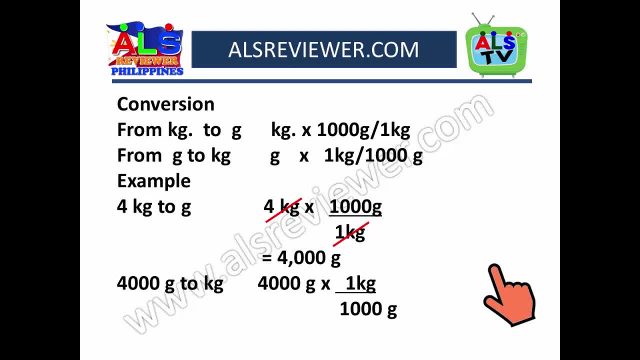 Or it means dividing, I should say Dividing 1,000 into divided by 1,000. Because 1 kilogram is equal to 1,000 grams. So mangyayari, dyan, Icocancel, out natin yung grams and grams. 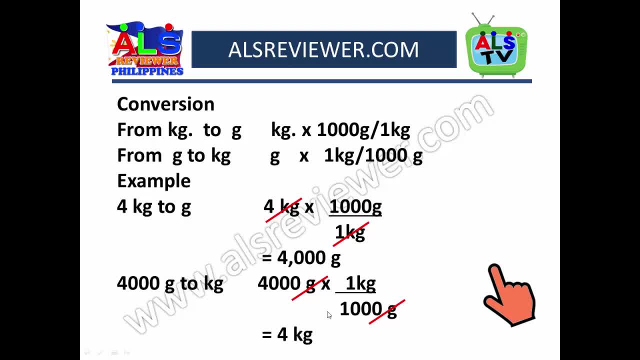 Ang natitira na lang yung kilograms Kaya ang sagot: dyan 4,000 divided by 1,000.. 4 natitira ng unit is kilogram, Kaya 4 kilograms. Okay, So tandaan lang. 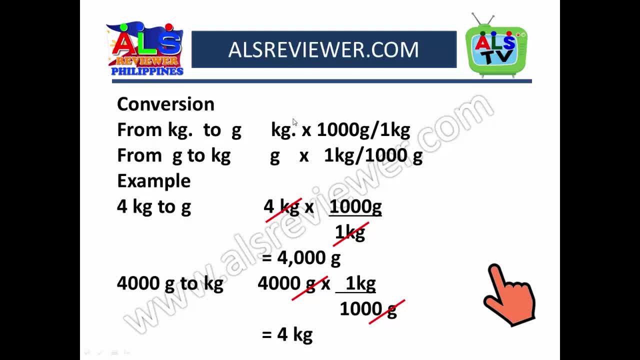 Pag malaking unit yun, Okay, Itatranslate natin ng mas maliliit na unit. Okay, I-multiply lang natin. Multiply, Multiply times 1,000.. Pag kayong maliit na unit, grams. 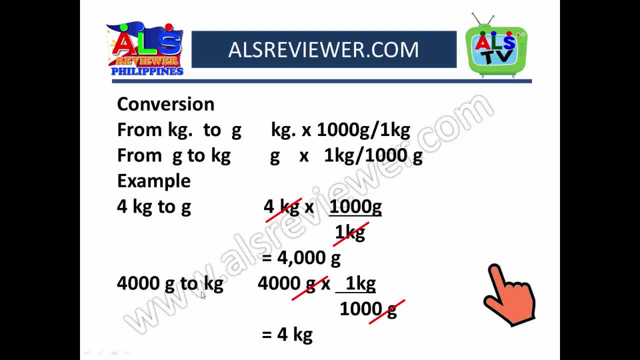 Okay, Icoconvert natin sa bigger units. Alright, I-didivide lang natin sya ng 1,000.. Let's go to the next, From kilograms to grams. Example Alimbawa: 34 kilograms to grams. 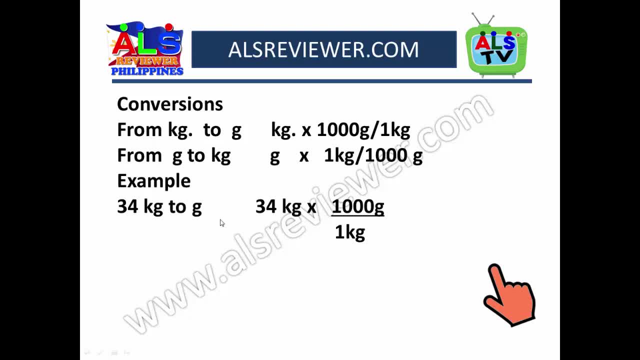 Paano natin i-coconvert yung 34 kilograms. So 34 kilograms times Ibig sabihin Itatimes lang natin ng 1,000.. Okay, So ang ginamit natin is 1,000 gram over 1 kilogram. 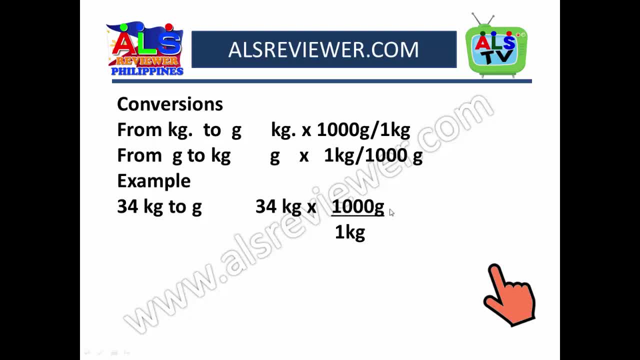 Because this represents that in 1 kilogram there are 1,000 grams. So presenting the equation like 34 kilograms to 1,000.. Okay, So 34 kilograms to 1,000.. Okay, So presenting the equation like 34 kilograms times 1,000 gram over 1 kilogram. 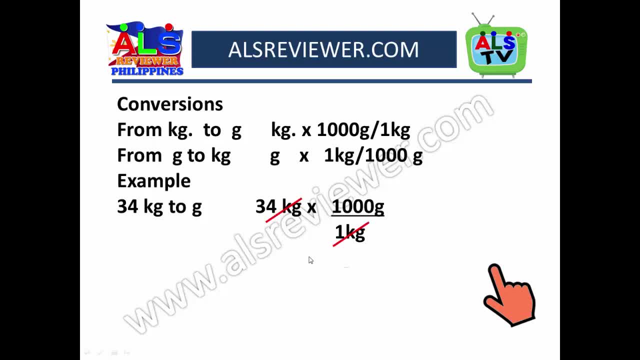 So that we can cancel out, Cancel out kilograms there, And then we multiply 34 by 1,000 is 34,000.. Ang natitirang unit is grams. That's why 34,000 grams, Okay, Yung 34,000 grams naman, kapag kaibalik natin sa kilogram. 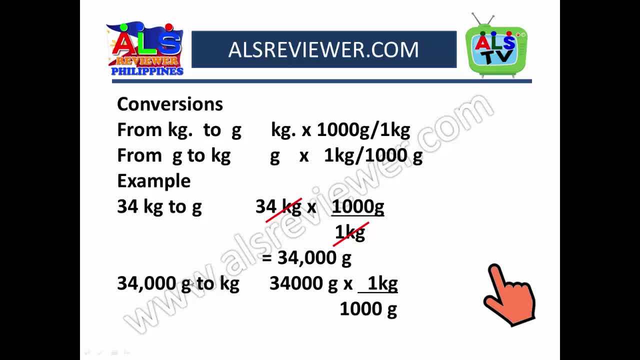 Okay, So ang gagawin lang natin: Smaller unit. Smaller unit yung grams, Yung value na lumalabas Parang ang laki, Kasi smaller units yung binilang natin Ngayon dito. 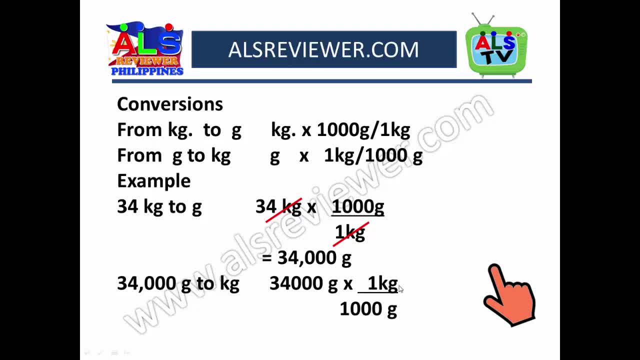 34,000 grams times 1 kilogram over 1,000.. So ang sagot nyan- Ika-cancel out natin yung grams- Ang magiging sagot is 34 kilograms. Bakit naging 34?? 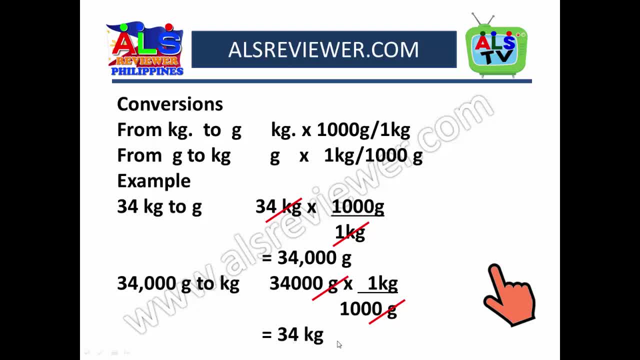 Kasi 34,000 divided by 1,000.. That becomes 34.. Okay, So I hope naintindihan na natin kung paano tayo mag-convert. Okay, Ito naman Another example pa. 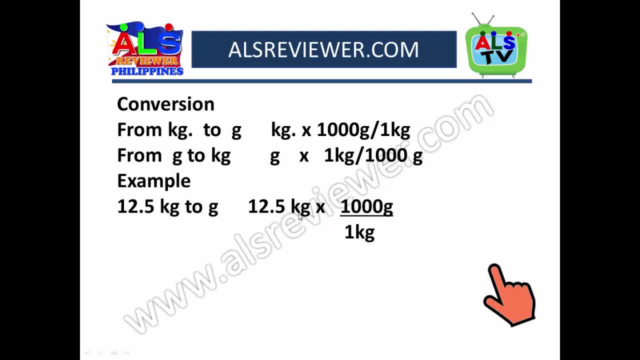 12.5 kilograms to grams. Ang gagawin lang natin: From kilograms to grams, Mumultiply natin ng 1,000.. Kaka-cancel out yung kilogram. Parang matitira ay grams Yung unit. 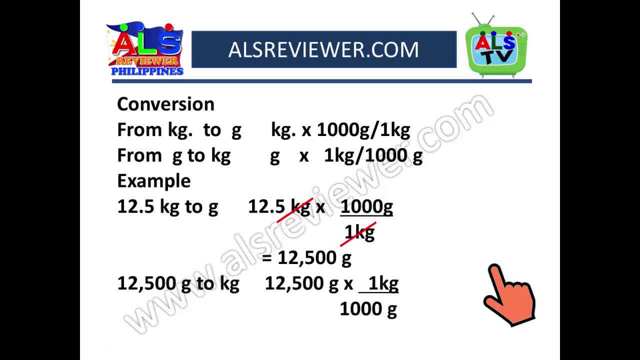 Okay, That's 12,500 grams. Alright, Pag 12,500 grams Ibabalik natin sa kilogram Halimbawa, That's 12,000 grams times 1 kilogram over 1,000.. 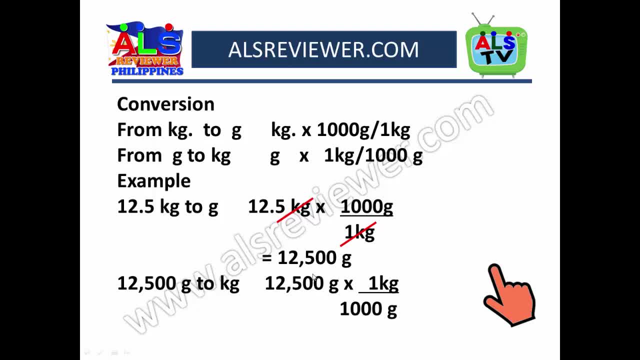 Or ibig sabihin lang nito: Ang presentation na to Ang nakikita nyo is times, Pero actually ang ginagawa natin is 12,500 divided by 1,000.. Okay, So magiging sagot nyan. 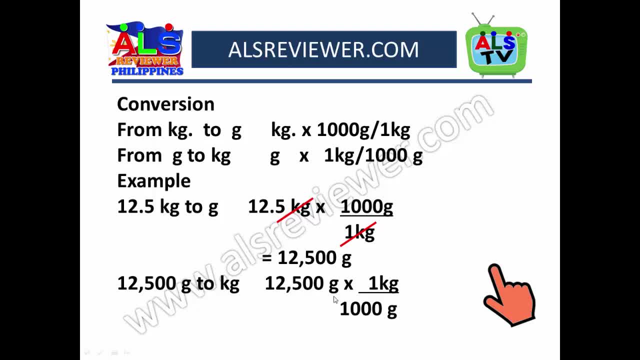 Cancel out the grams. Ang natitira is 12.5 kilograms. Okay, Let's move on. Ayan, Mayroon tayong mga steps to follow in solving math problems. Okay, Yung una Ito Ito. 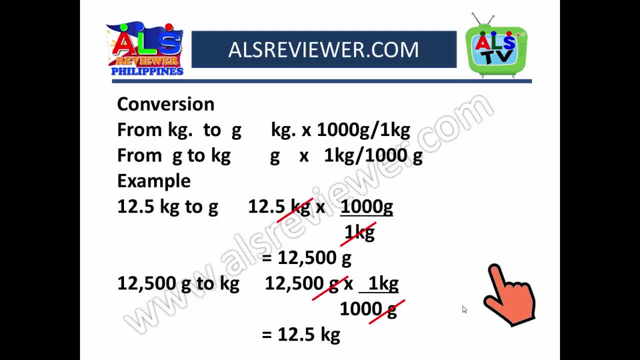 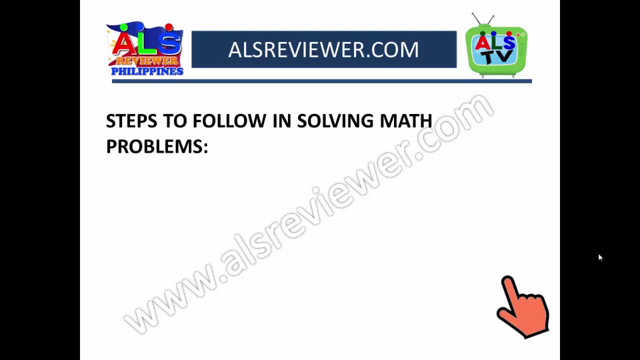 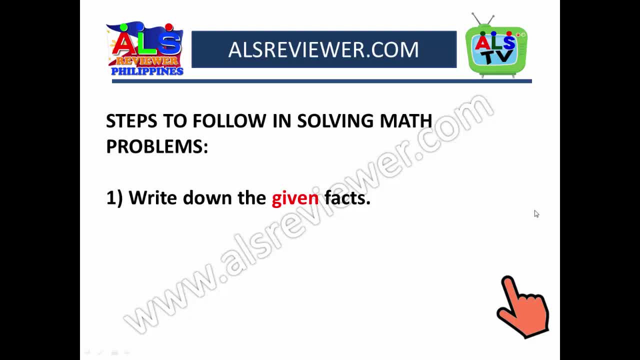 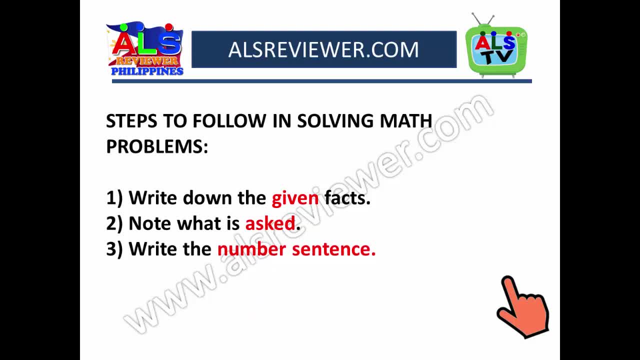 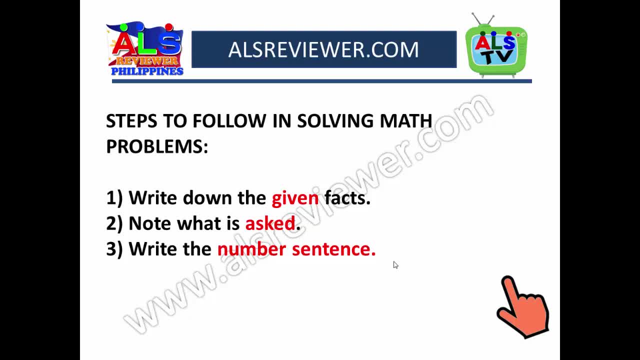 Yung 1 plus 1.. 1 plus 1 equals 2.. Yun na yung magiging number sentence. Okay, tingnan natin. mamaya, Show your solution. Solution, ibig sabihin kung paano mo na ito i-solve. 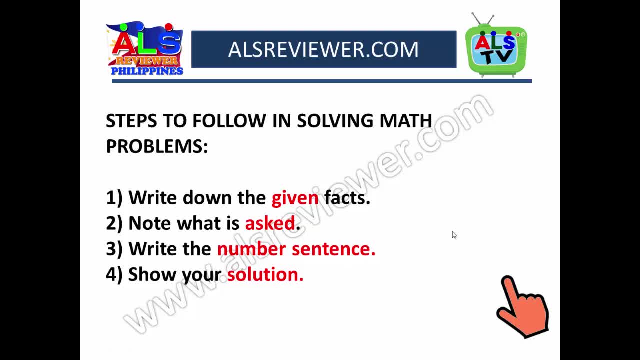 Applying yung different operations. ano yung gagawin mo: Mag-a-add ka ba, Mag-subtract, Mag-divide Or mag-multiply Ayan. so ipakita mo ngayon yung solution mo, And then number 5, make a conclusion. 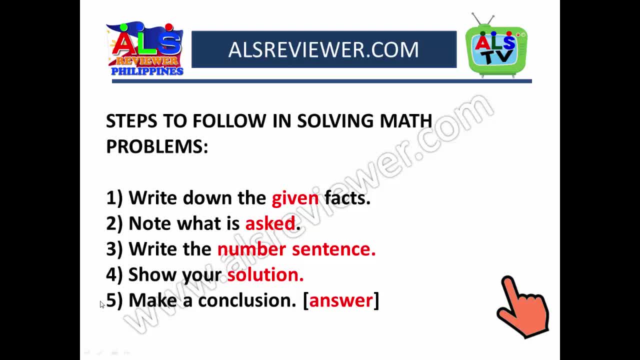 Ano ngayon ang sagot mo? yung answer: Usually ang number 5 is sinasagot niya yung what is asked in the problem. Kung alam natin what is asked, kukunin natin ngayon dito dun sa make a conclusion. yung answer. 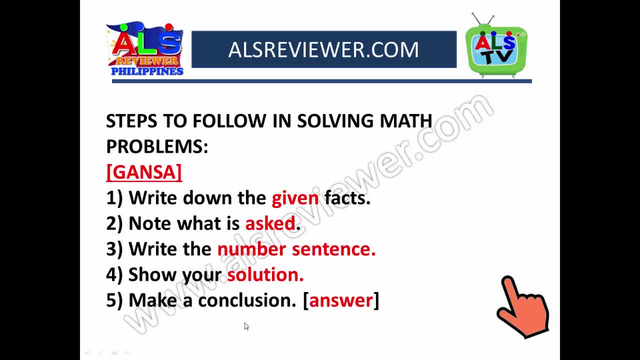 Sasagutin nito, yung number 2.. Okay, So meron akong abbreviation na ginagamit para hindi ninyo makalimutan yung arrangement nito at, kung ano-ano, yung mga isusulat ninyo. 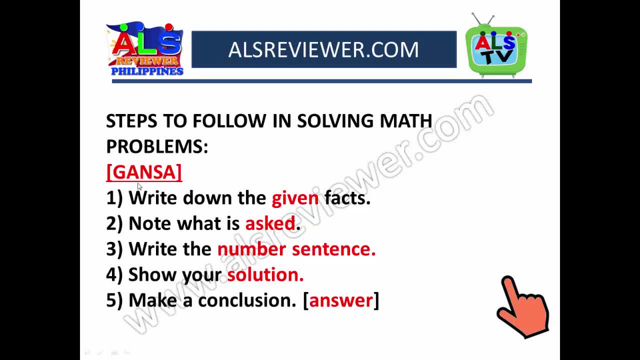 At ang acronym na yan is GANSA Yung GANSA, ibig sabihin G is given, A is ask, N is number sentence, S is solution, A is answer. Para madaling maintindihan, madaling ninyong ilagay sa isip kung ano yung mga kailangan, yung steps na sundin kapag nagsosolve kayo ng problem. 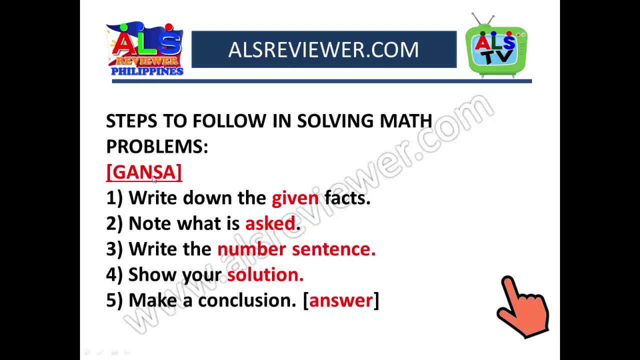 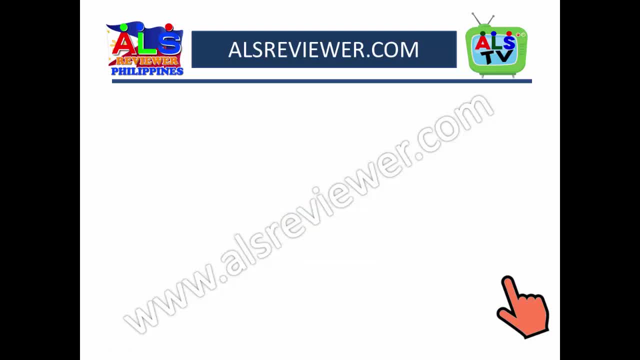 GANSA, Okay. So given ask number sentence solution and answer: Okay, We're going to apply this one later on. Ia-apply natin ito, mamaya, Okay. So halimbawa ito yung problem natin. 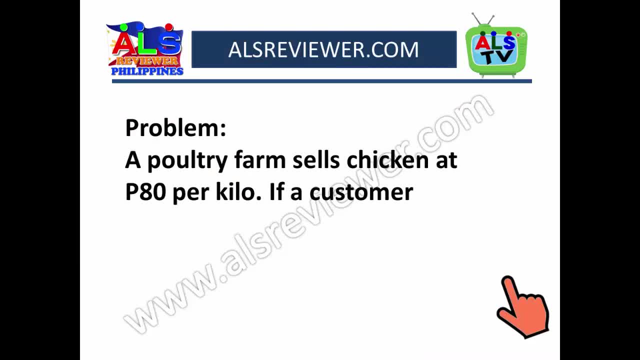 A poultry farm sells chicken at 80 per kilo. If a customer bought 4,800 pesos worth of chicken, how many kilos did he or she buy? Okay, So ito yung problem natin. Tingnan nyo maigi kung ano yung mga given facts dito sa problem. 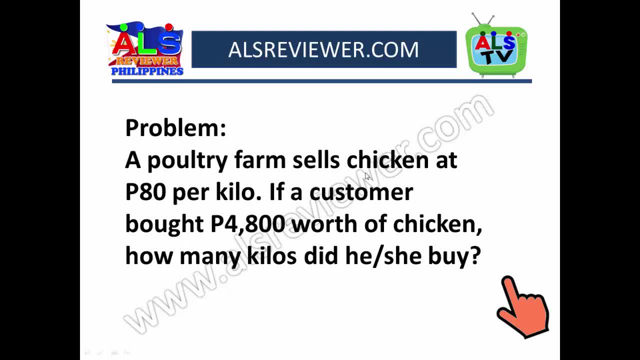 Meron tayong 80 pesos dito, So ano yun Per kilo of chicken And then 4,800 dyan yung worth of chicken na binili ng customer. Ngayon titignan natin yung question nya. 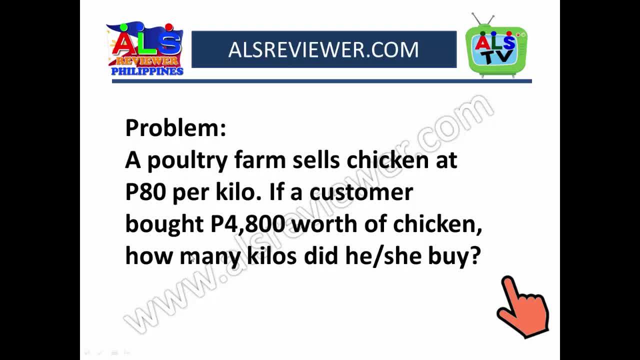 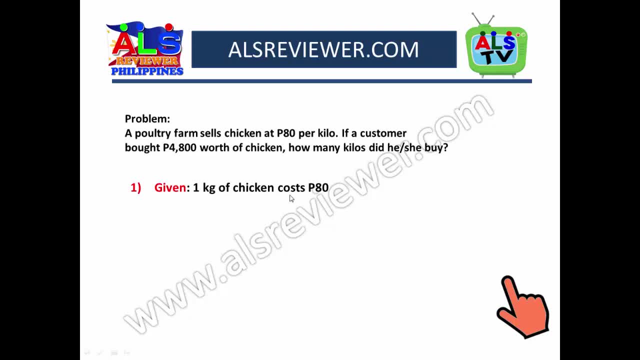 How many kilos did he or she buy? So ang hinahanap natin kilos, Apply natin yung steps. Okay, One given is one kilogram of chicken costs, Ah, 80 pesos. Okay, Yun yun. 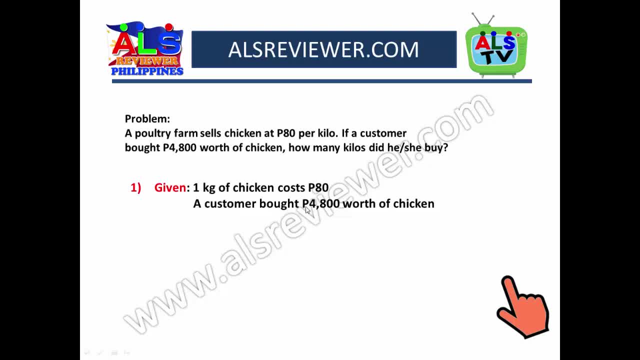 Yung number two naman, yung susunod pang given is a customer bought 4,800 worth of chicken. Okay, So alam na natin yung mga given. Punta na tayo dito sa ask. 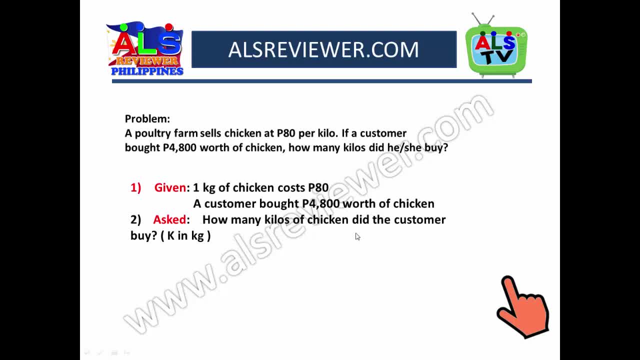 What is ask? Ano, yung tinatanong sa problem: How many kilos of chicken did the customer buy? Variable K, which is in kilogram, Okay, Tinan natin Ang number sentence natin. Tinan natin ngayon: kung K ito okay, 80 pesos times, kung ilang kilo, ang binili nya ay magiging 4,800. 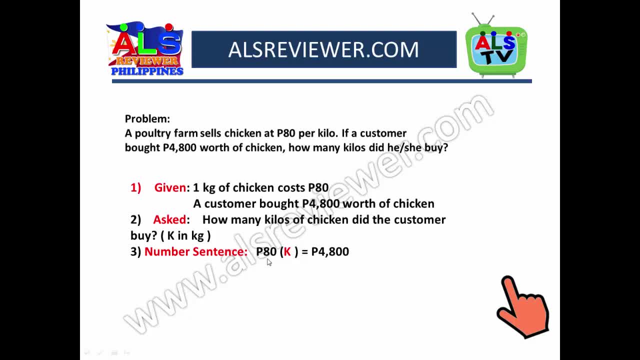 Yun yung pinambayan nya. So ito ngayon yung number sentence natin: 80 pesos times the unknown number, which is the number of kilograms, is equal to yung pinambayan nya: 4,800.. 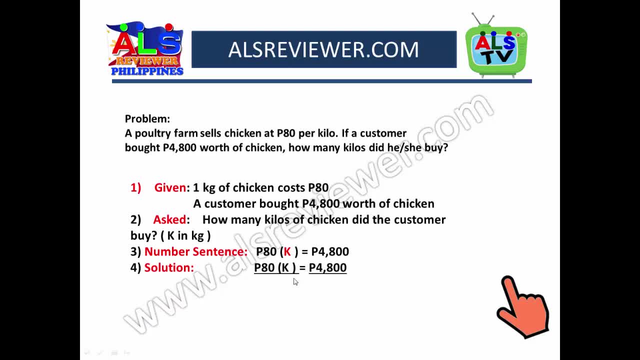 So yan yung number sentence. So ito ngayon yung solution natin: 80 pesos times K is equal to 4,800.. Ang nga gawin lang natin, ang dapat malaman natin yung K. 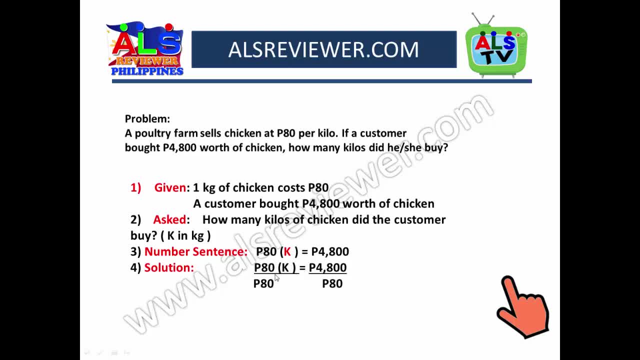 So dahil equation ito: i-eliminate natin yung 80, aalisin natin yun para matitira lang K At para maalis yung 80 dito kailangan lang natin i-divide ito. 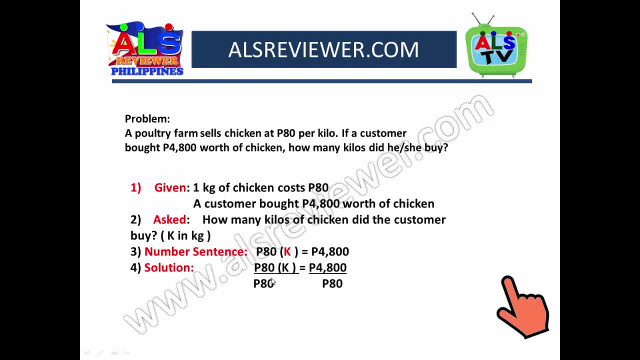 Both sides of the equation i-divide natin ng common number. okay, So para maalis, talaga ito yung 80, ang ipandivide natin 80 pesos At dito sa kabila naman 80 pesos din. 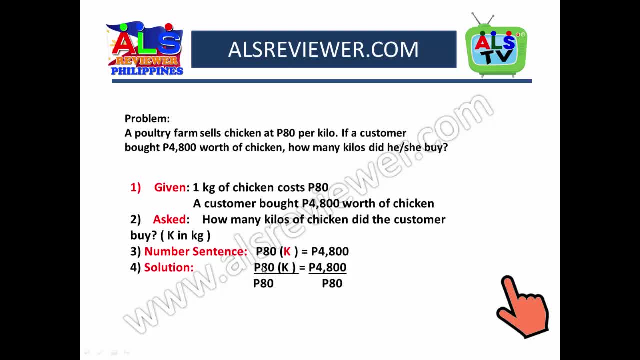 Ang ipandivide natin. So anong gagawin natin, Pag na-divide na natin ito, that cancels out? Wala na siya, Kasi 80 divided by 80, magiging 1 na lang siya. 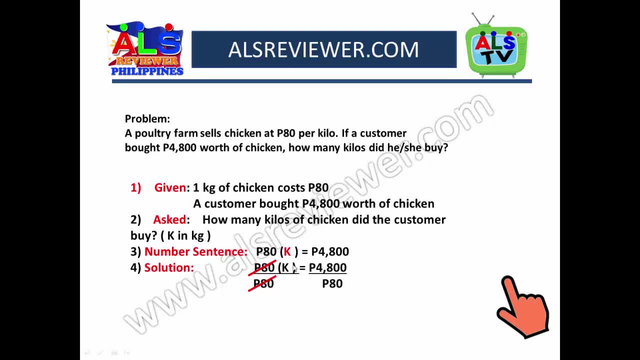 1 times K. Kung ano man yung value ng K, yun pa rin ang lalabas. Kaya eliminated na yung price Dito. sa kabila naman 4,800,. i-divide natin sa 80.. 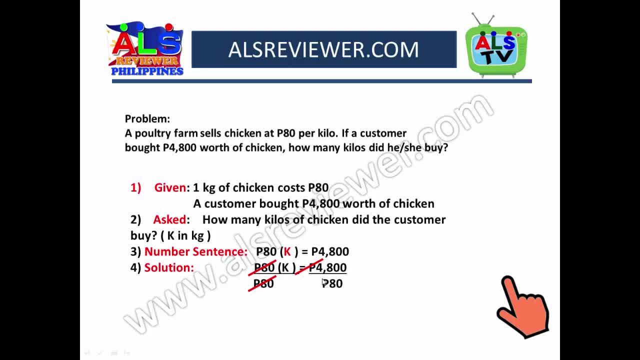 Okay, Pero aalisin na natin yung Units which is pesos, Aalisin na yung unit niya sa. natitira na lang yung unit ng K, which is kilogram. Okay, So ang K ngayon equals 60 kilograms. 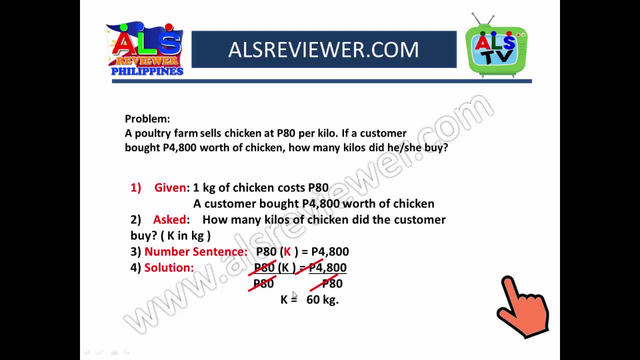 Okay, So napaka ganda na alam natin kung papaano tayo, anong mga ginagawa natin, para alam natin kung ano yung unit na lalabas dun sa answer, Kasi kapag nagkabalibalig talaga, 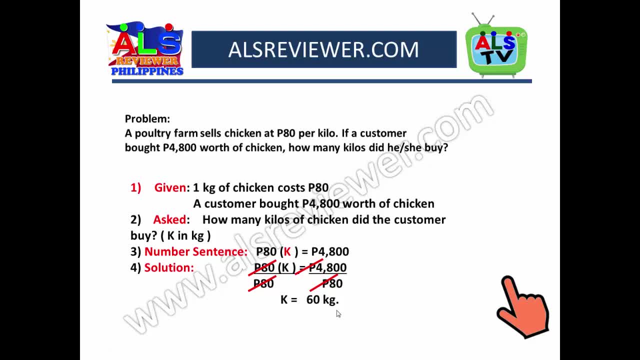 yung mga numbers, ibig sabihin magkabalibaligtad din kung saan natin iligay yung mga units, at hindi magiging tama yung sagot natin. Okay, So tapos na natin ang solution. 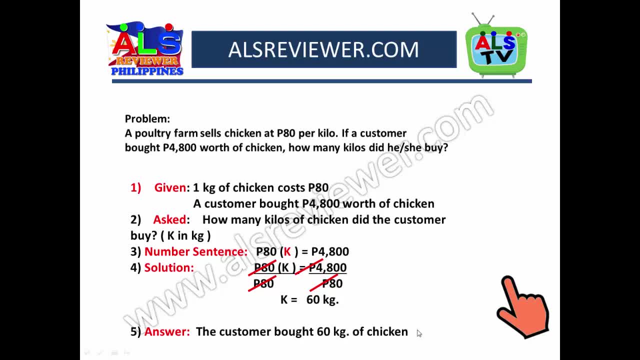 Ang answer natin: the customer bought 60 kilograms of chicken. Ito na yung sagot natin. from the solution na ginawa natin, Isasagutin na natin ngayon. yun what is asked: How many kilos. 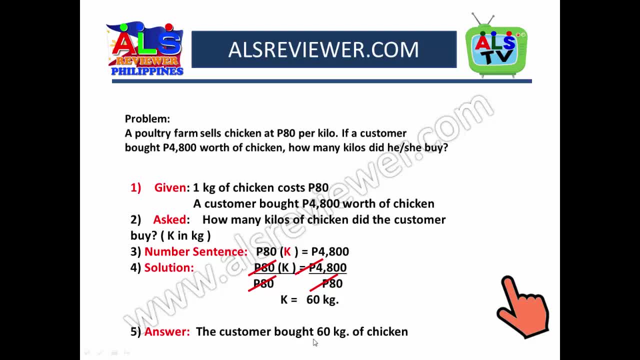 So ang hinahanap kilos Kaya naman dito sa answer natin, customer bought 60 kilograms of chicken. Okay, So we have properly applied these steps in solving problem, at saka yung acronym natin kanina na GANSA. 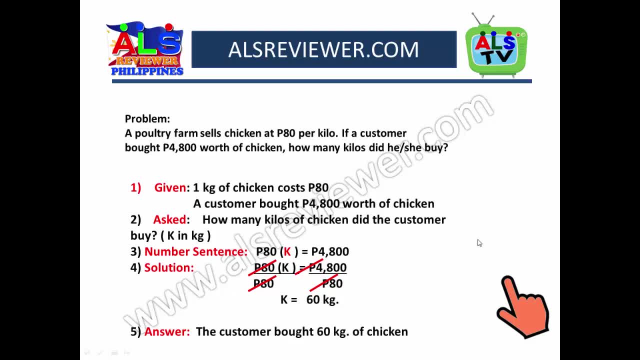 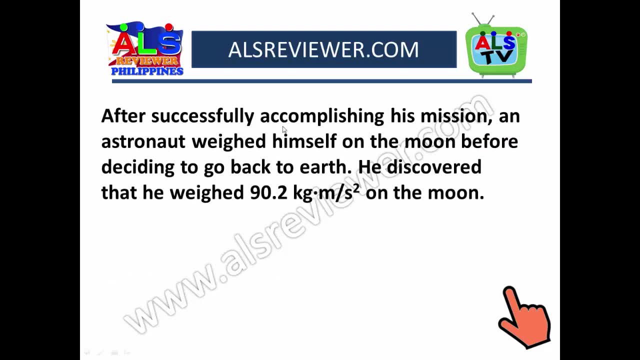 Given ask number, sentence solution and then answer: Okay, Let's try another one. Ah, this is another problem. After successfully accomplishing his mission, an astronaut weighed himself on the moon before deciding to go back to Earth. He discovered that he weighed 90.2 kilogram meter per second squared on the moon. 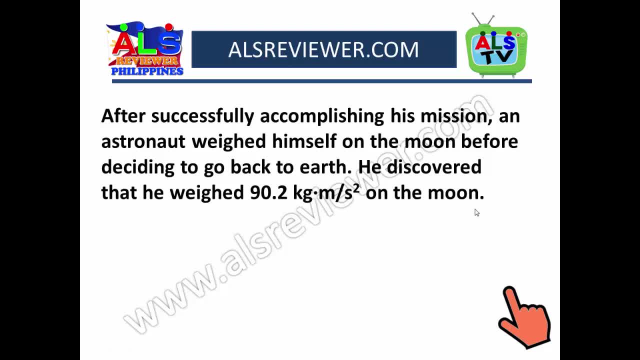 So bakit natin tinitingnan yung weight nung astronaut dun sa moon at saka dito sa Earth? Pag ibabalik natin dun sa video, Yung weight is being affected by the. Yung weight is being affected by the. 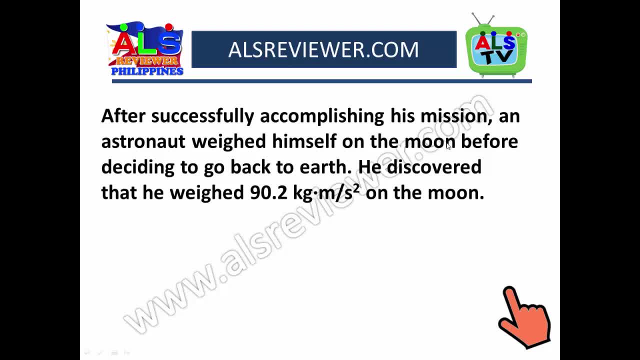 Yung weight is being affected by the, by the pull of gravity on the moon. Ito yung weight ngayon ng astronaut. Okay, 90.2 kilograms meter per second squared. Titignan natin kung ano yung tinatanong ng problem. 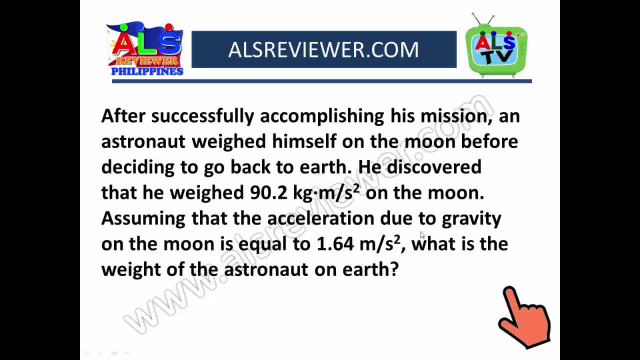 Ano ba yung tinatanong problem? Assuming that the acceleration due to gravity on the moon is equal to 1.64 meters per second squared, Ito yung acceleration. Ito yung acceleration due to gravity. Yung hila ng gravity sa moon is 1.64 meter per second squared lang. 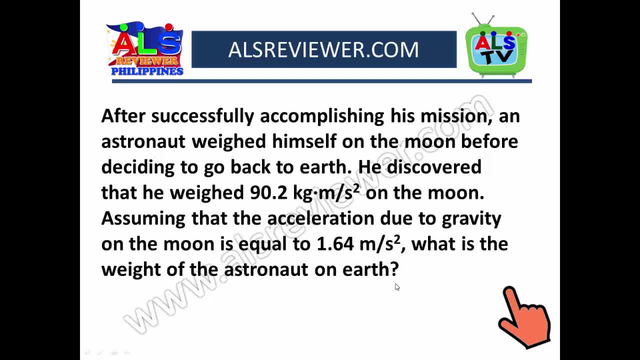 What is the weight of the astronaut on Earth? So ikukumpira ngayon natin yung bigat ng astronaut dun sa buwan at saka yung bigat niya dito sa lupa. Okay, So tingnan natin kung paano natin ito sasagutin. 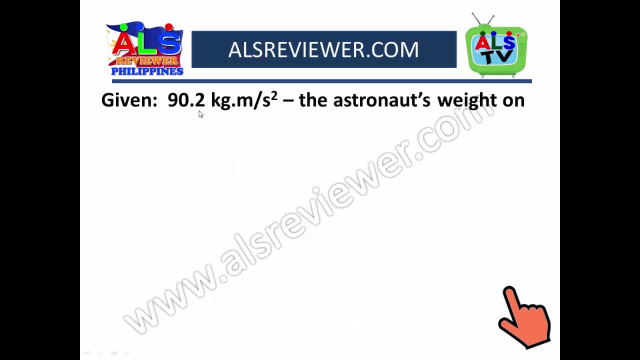 So ang given facts natin Given is 90.2.. 2 kilograms meter per second squared The astronaut's weight on the moon. Ito yung bigat niya. Okay, Ngayon ang pull of gravity on the moon is 1.64 meter per second squared. 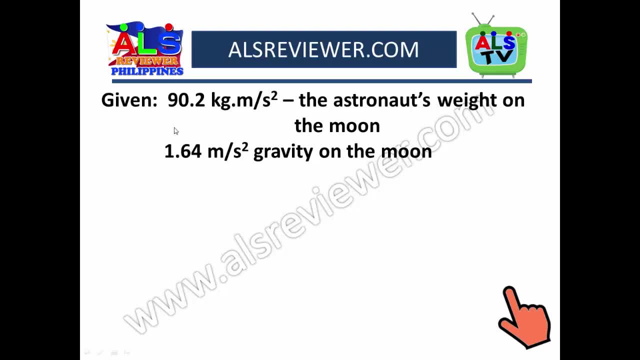 Kung baga ito yung lakas ng hila ng buwan dun sa katawan ng astronaut, Okay, Ngayon naman hindi ito given, Pero alam natin dun sa problem hindi ito na ibigay. 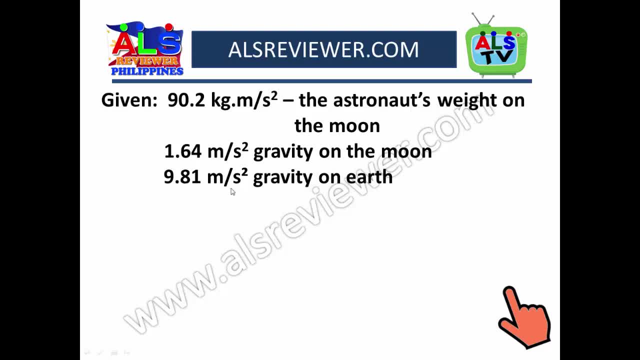 But we know, because this is a constant, that 9.81 meter per second squared is the pull of gravity on Earth. So kailangan mayroon din kayong stock knowledge on the values of the gravitational pull. Ito, yung constant ngayon dito sa Earth is 9.81 meter per second squared. 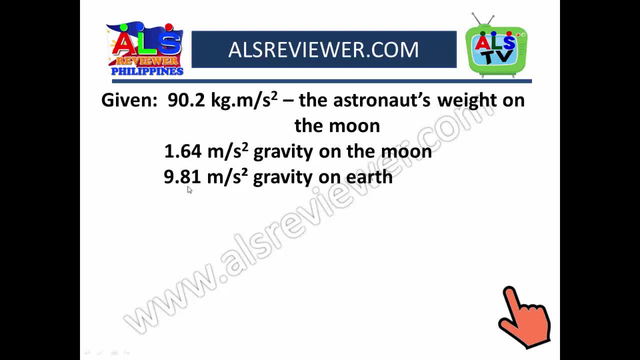 So pag i-compare natin dun sa gravity, pull of gravity on the moon, Talagang napakalakas dito sa Earth Napakahina dun sa moon Ask. So alalahanin ninyo yung gansa given. 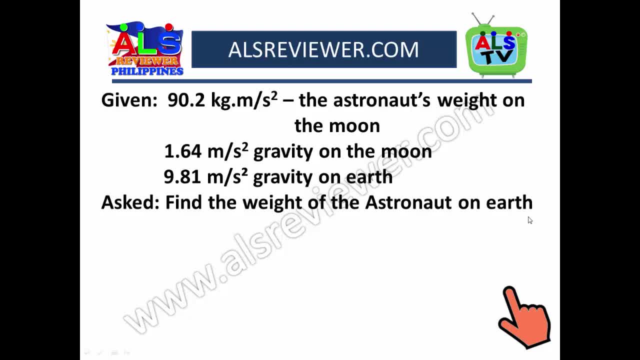 Ask: Find the weight of the astronaut on Earth? Ito yung kinatanong. Pero meron tayong hidden question, Yung hidden question: what is the mass of the astronaut? Kasi alam natin na yung formula is: weight is equal to mass. 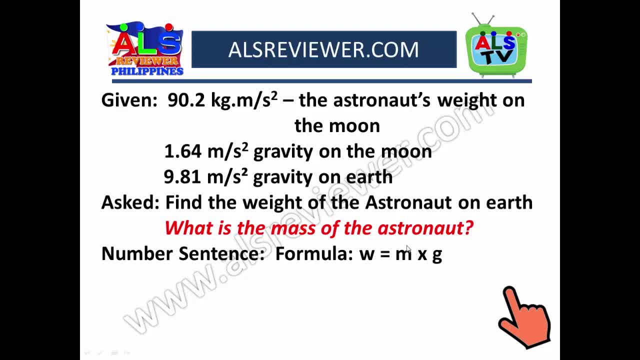 Times gravity, Pero hindi natin alam yung mass. Hindi natin alam kung ano, yung gaano kalaki yung katawan ng astronaut. Alam natin yung kanyang weight O kaya bigat sa buwan na naapektuhan ng gravitational pull which is 1.64 meter per second squared. 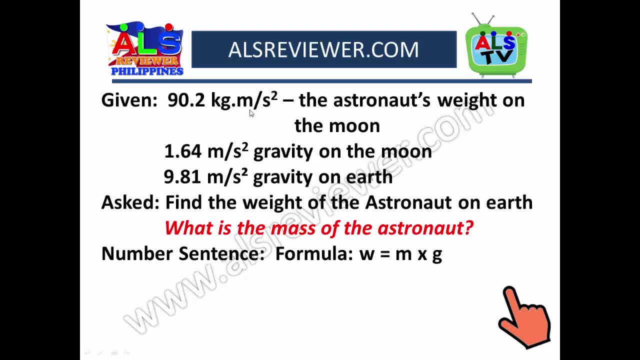 Alam natin yung weight, which is 90.2 kilograms meter per second Squared. Alam natin yung pull of gravity, which is 1.64 meter per second squared, Pero hindi natin alam yung mass. 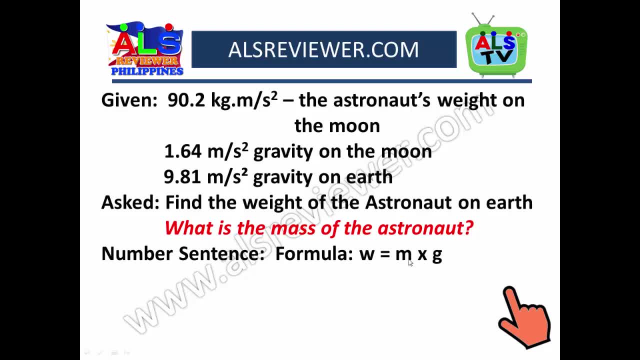 Okay, Kasi bakit natin kailangan kunin yung mass? Kasi yung mass or yung bigat ng dami ng elements ng katawan ng astronaut is hindi yung nagbabago Yung dami? 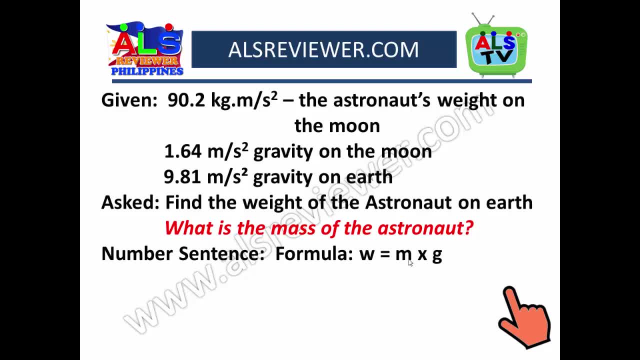 O yung gaano siya kalaki, Hindi yung nagbabago sa buwan at sa lupa, Kaya parehas lang yung mass niya dito. Okay, Ang nagbabago kasi yung weight, dahil affected siya dun sa pull of gravity on the moon at saka yung pull of gravity on the earth. 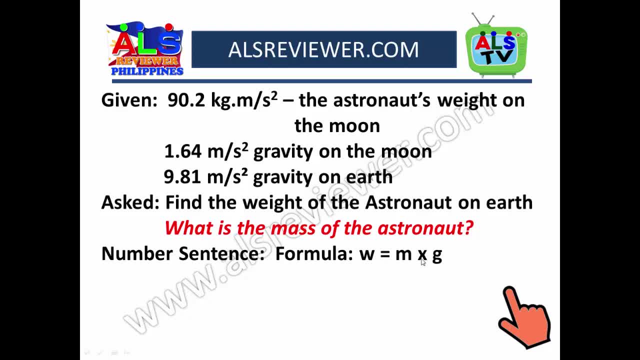 Okay. So ang number sentence natin, formula, is: weight is equal to mass times the gravitational pull. Okay, Where yung mass? Eto na yung sinasabi, Sinasabi natin Paano natin kukunin: yung mass is equal to weight over the gravitational pull. 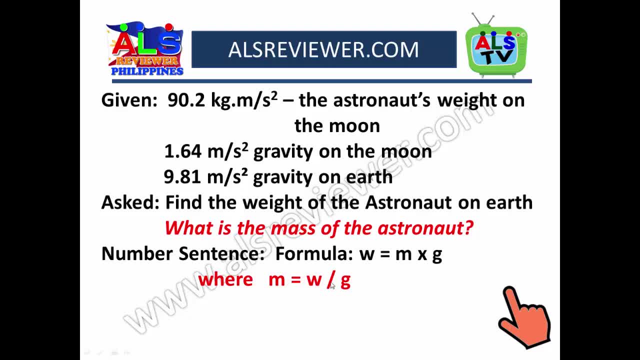 Bakit? paano yun nangyari? Bakit mass is equal to weight over gravitational pull. Kasi kung i-transmute natin itong, formula ng W is equal to N times G. ang gagawin natin dito? 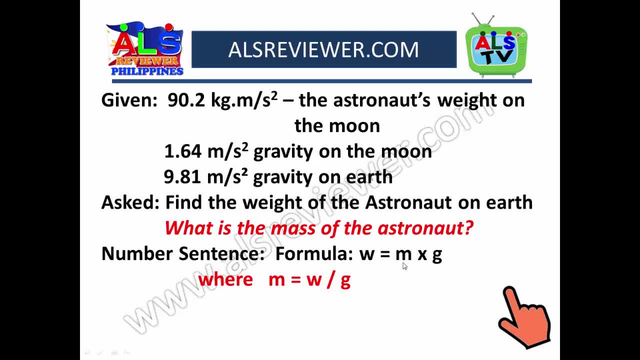 i-divide natin yung both side of the equation para matira lang yung. So i-divide natin ito ng G. I-divide din natin sa kabila yung W ng G. Pag kinunsel out natin yung dalawang G, ang natitira na lang M. 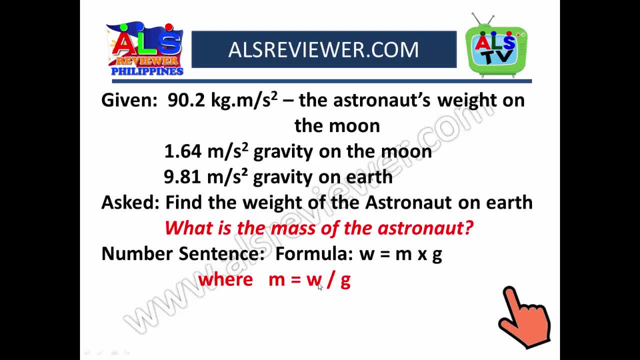 So W over G, Kaya M mass is equal to W over G. Okay, So alam na natin, Alam natin ngayon na yung mass is equal to weight. Okay, Over the gravitational pull. So weight is 90%. 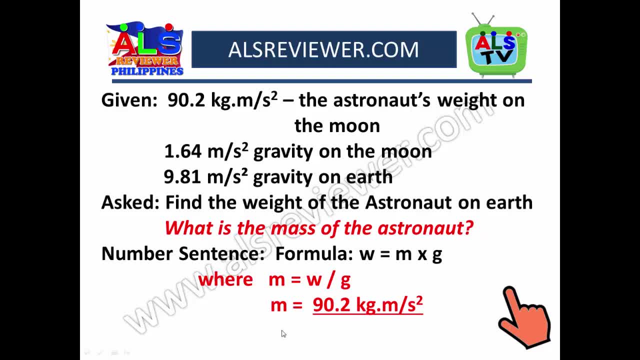 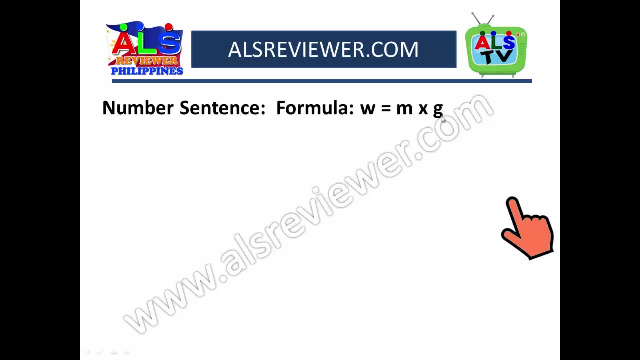 So weight is 90.2 kilograms. Okay, So alam natin na yung G, which is 1.64 meter per second, squared Okay Number sentence natin. So yung formula natin, W is equal to M times G. 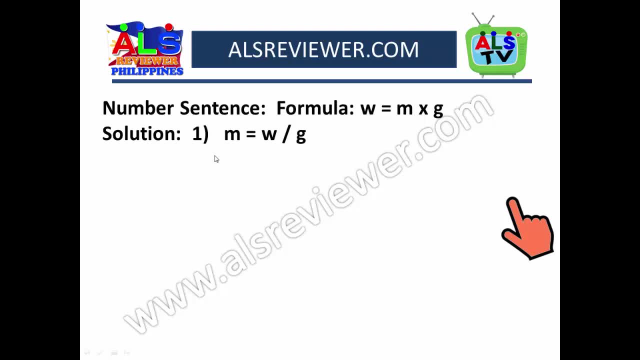 Okay, And then ang solution natin Okay. Meron tayong dalawang solution: Una yung paghanap natin ng mass Okay. So tingnan natin Solution natin Okay. Solution number one: 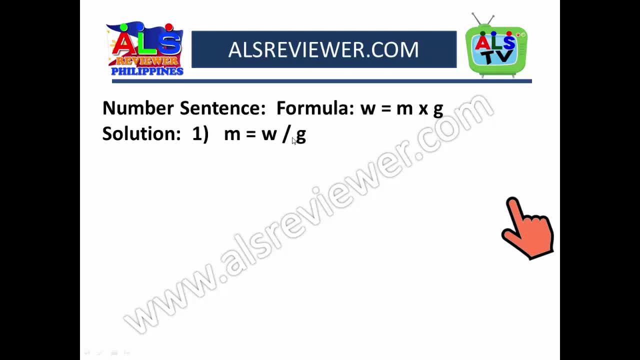 Hanapin muna natin yung mass, kasi hindi pa natin alam. So mass is equal to W over G. So kanina nakuha natin. Okay, Cancel out natin yung meter per second squared. 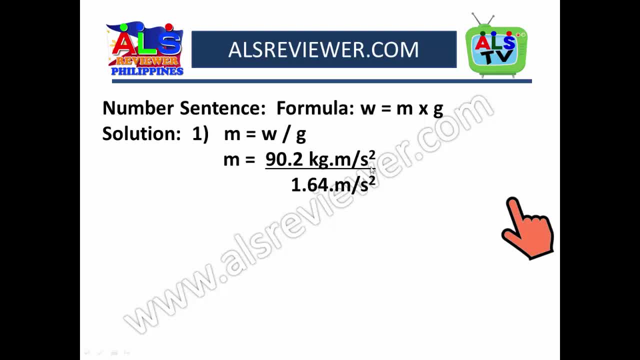 Meter per second, squared. Okay, Pwede natin i-cancel out ito. Okay, So ang magiging sagot is: meter or mass is equal to W over G, Equal to 55 kilograms. Okay, Dun tayo sa number two. 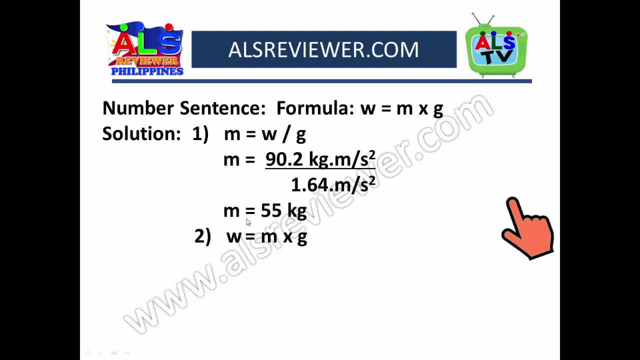 Ang number two solution natin, uplying the mass, which is 55 kilograms, Kasi hindi naman nagbabago itong mass na ito, Yung laki ng katawan ng tao sa buwan at saka sa lupa, hindi nagbago yung laki ng katawan nya. 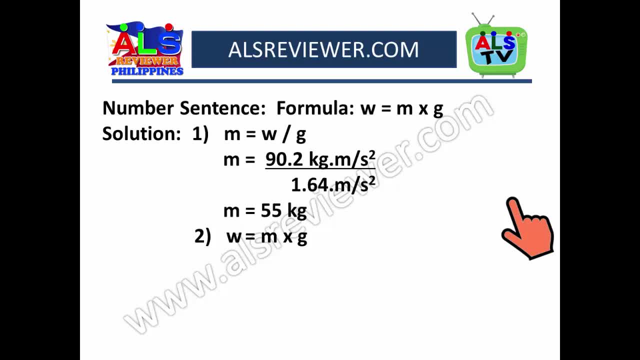 Kaya gagamitin nga yung natin, yung nakuha nating laki ng katawan, yung bigat ng laki ng katawan Okay, Which is 55 kilograms. It is to substitute natin ngayon sa formula: W is equal to M times G. 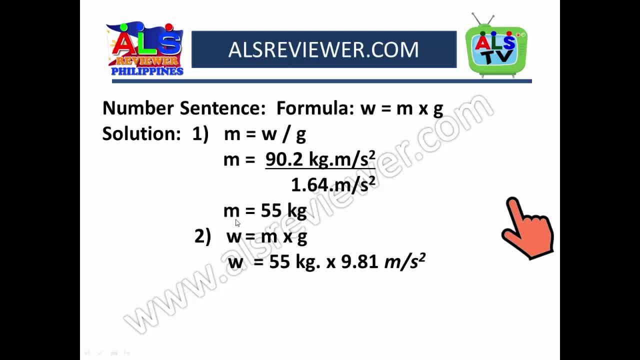 So ang gawin natin W is equal to 55 kilograms. yung nakuha nating mass times 9.81 meter per second squared. Ito naman ngayon yung G. yung G resists the gravitational pull of Earth on a body. 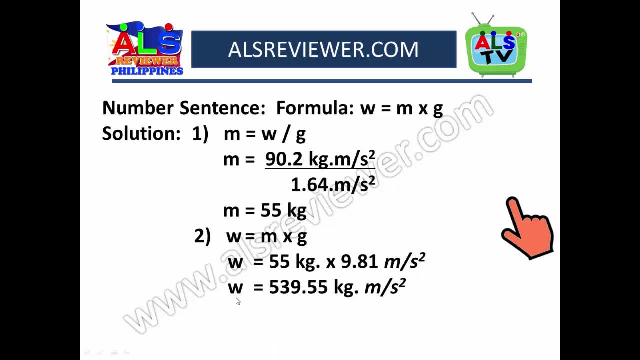 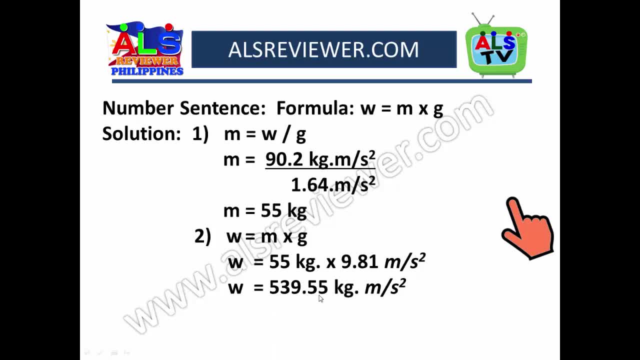 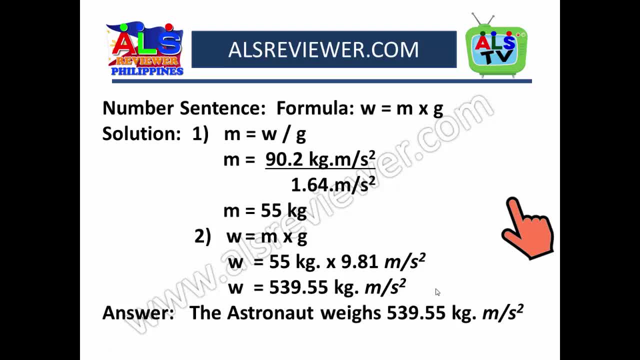 The astronaut weighs 539.55 kilogram meter per second squared. Ayun, So compared, Okay Compared dun sa bigat nya Dun sa buwan, which is ito: 90.2 kilograms meter per second squared. ito yung bigat nya sa buwan. 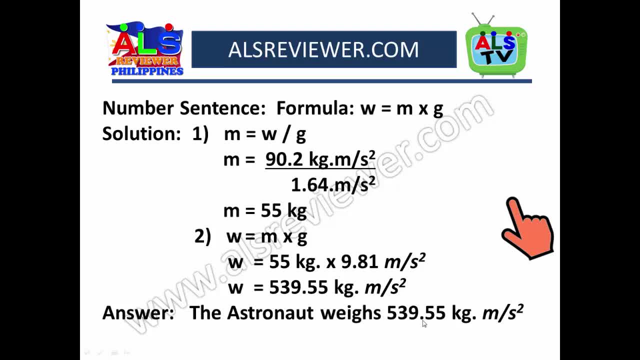 okay, eto naman ngayon yung bigat ng astronaut dito sa lupa affected by the pull of gravity, which is 9.81 meter per second squared. ang bigat nya ay 539 539 .55 kilograms meter per second. 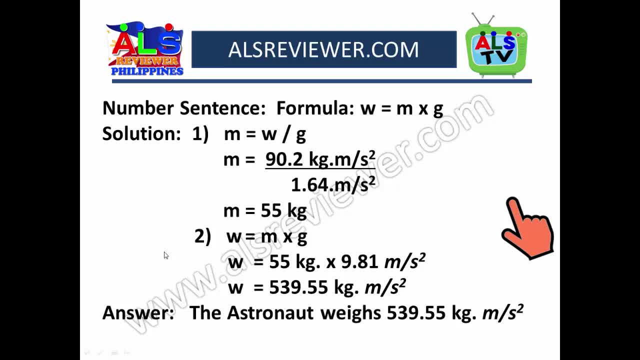 squared. okay, nasagot ba natin yung tanong: gaano kabigat yung astronaut dito sa lupa? okay, so eto ngayon. the astronaut weighs 539.55 kilograms. meter per second squared on earth. alright, so yan yung. 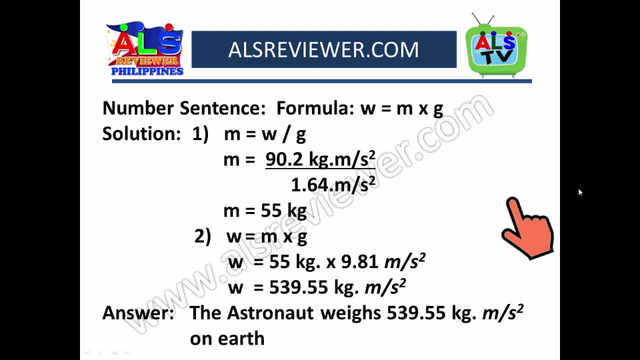 ating sagot dun sa problem na yun. okay, so tuloy-tuloy, tayo ay ayun kinancel out, so ito yung pag-cancel out dun sa unit na m per second squared. m per second squared para. 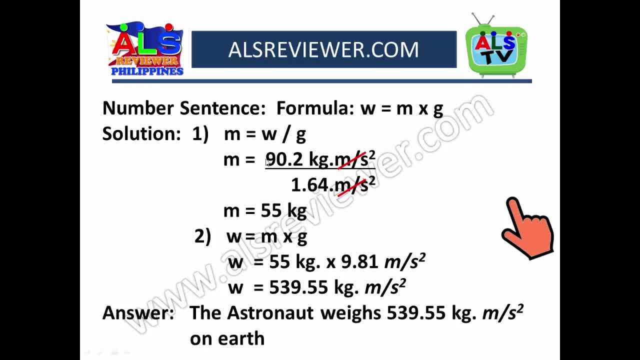 ang natitira lang. okay, ang natitira lang dito kanina is 55 kilograms, kasi ang unit na kilograms na lang ang natitira dito kaya, kilograms lang ang kanyang unit, okay, so let's, let's. 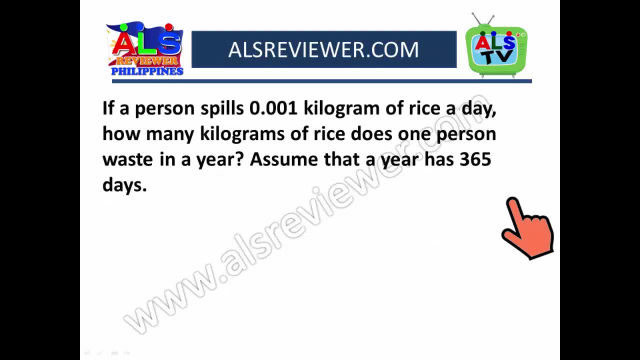 go ahead. another problem: if a person spills .001 kilogram of rice a day, ayun, how many kilograms of rice does one person waste in a year? assume that a year has 365 days. okay, so ano ang tinitingnan natin, tinitingnan natin gaano ba. 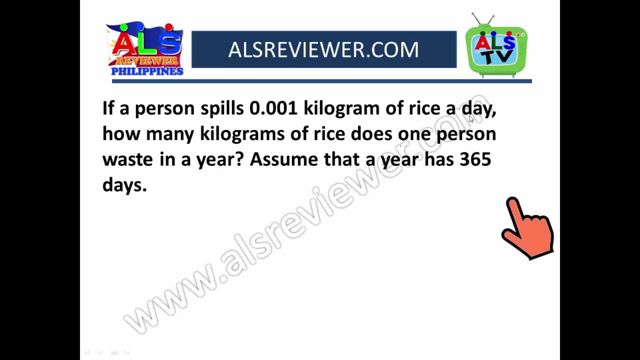 karaming kanin ang nasasayang ng isang tao sa isang taon kung ang and kanyang natatapon ninguna is point, zero, zero, one kilogram. ibig sabihin siguro, medyo sabihin na natin: 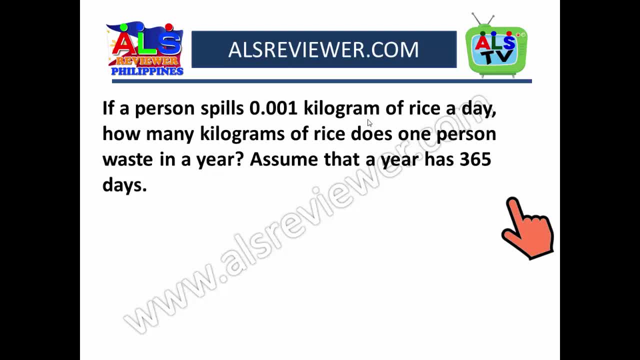 ighty sampung botil ng kanin. ito nawawala, natatapon sa sahig kalimbawa. okay so, titignan natin ngayon gaano ba karami isang tao ng pinag-uusapan na. 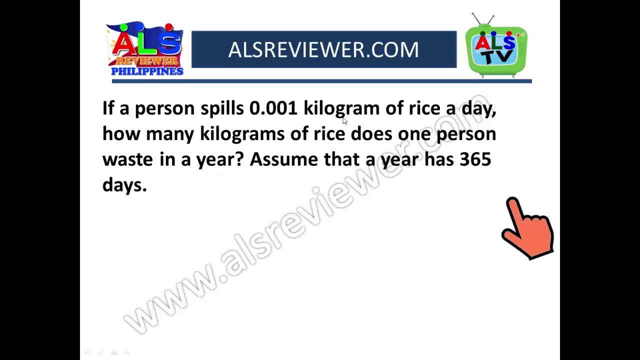 Kapag hindi tayo Masinop dun sa pagkanin ng però kain, kapag burara medyo maraming, maraming natatapon na kanin, eto ngayon ang titignan natin. so ito yung ating acronym dun sa steps in solving problem: gansa. okay, madaling tandaan. 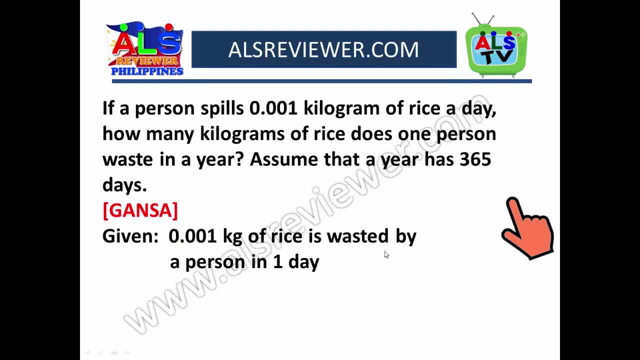 g. okay, given .001 kilogram of rice is wasted by a person in one day sa isang araw at there are 365 days in a year, so itong dalawang to ang given information na makakatulong sa atin sa pagsagot natin sa problem. okay, eto naman ang tinatanong: ask how many kilograms of rice is? 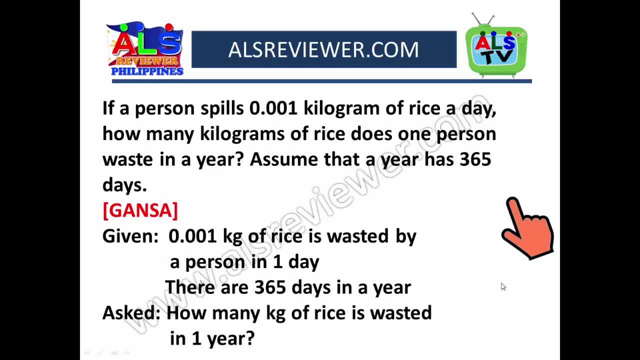 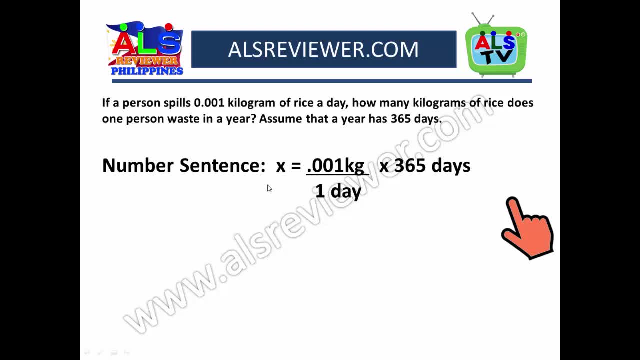 wasted in a year. gaano ba karami ang nasasayang sa isang taong. okay, ang number sentence natin. okay, i-re-represent natin. yung. gaano karami ng x. okay, x ngayon, pero yung X ngayon, dahil dami ng bigas ang pinag- uusapan. ang magiging unit nito is kilograms. ano po kilograms. 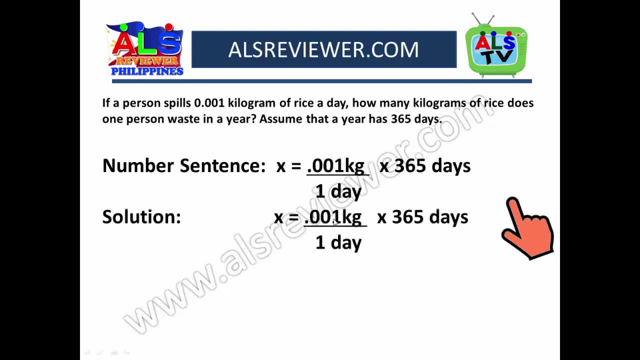 na anything na natin kong papaano natin makuha. bakit kilograms? kasi nga ang solution natin x is equal to .001 kilogram over 1 day times 365. si ang gagawin natin, alisin natin yung day or days, okay, pwede natin i-cancel ang day, the days, okay, pwede natin i-cancel, or do that. allora, bakit ang nellung day ka na to ay mayung managing 2st day king, eh. 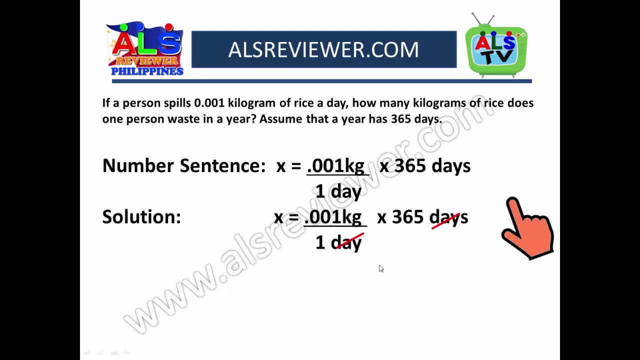 out. yan kasi parehas na unit araw, ang pinag-uusapan dyan. so ang natitira lang na unit is kilogram. so ang imumultiply lang natin itong number na to, as ako itong number na to nakuha na. 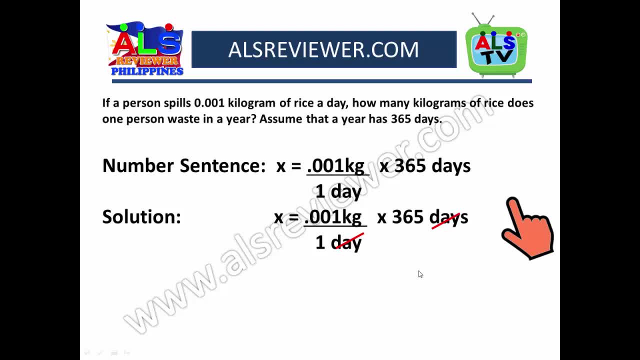 natin yung, kung ilang kilogram ang nasasayang sa isang taon. so tingnan natin to x is equal to 0.365 kilogram. kung, pag titignan natin 0.3 is one third of a kilo, okay, so yung ganun. 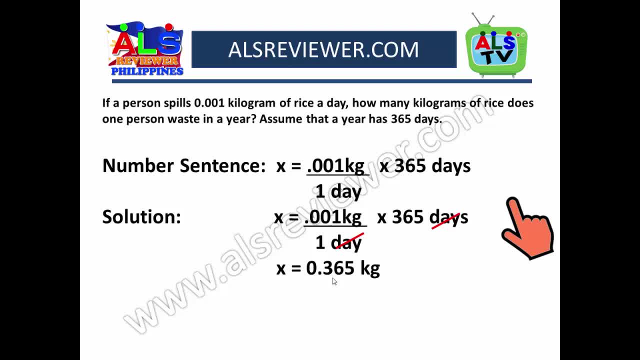 kadami yung nasisirang bigas sa isang taon, kapag ka ang natatapon is 0.001 kilogram, kumbaga isang kumpol ng kanin kasing laki siguro ng ating hinlalaki ayun. 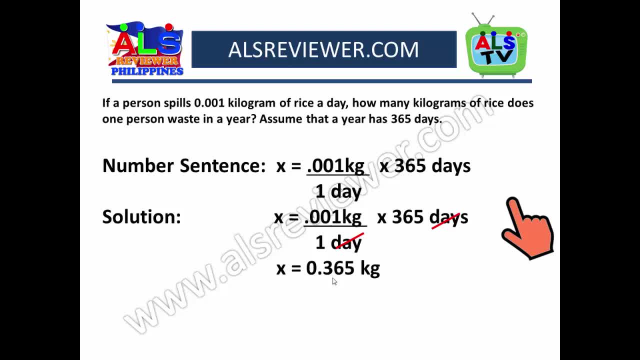 sa isang taon, o mas maliit naman siguro, sa isang taon, is 0.3, one third, one third of a kilo. yung nasasayang na ng isang tao lang. ayun, mga kaibigan, so yun yung solution, natin, yung answer. 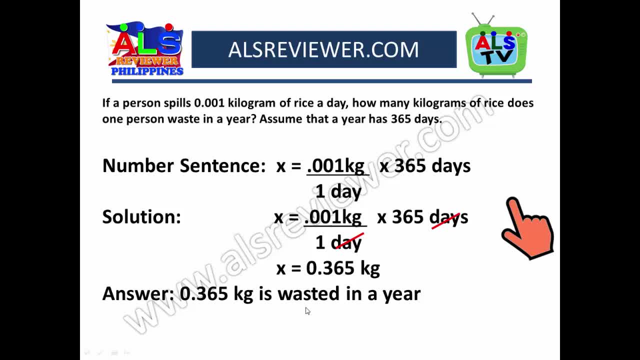 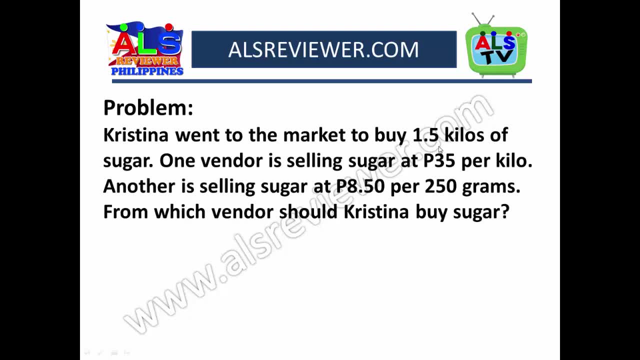 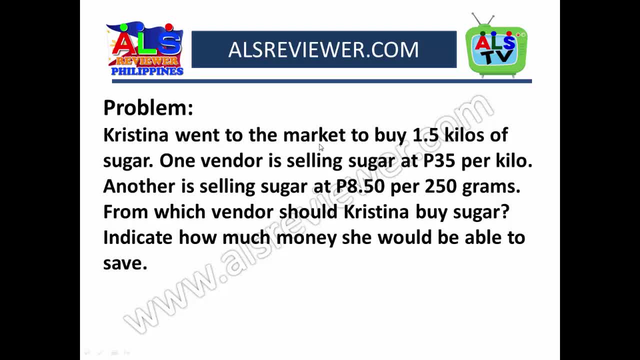 ito yung karugtong pala ng problem. ok, ulitin natin. Christina went to the market to buy 1.5 kilos of sugar. one vendor is selling sugar at 35 pesos per kilo. another is selling sugar at 8.50 per. 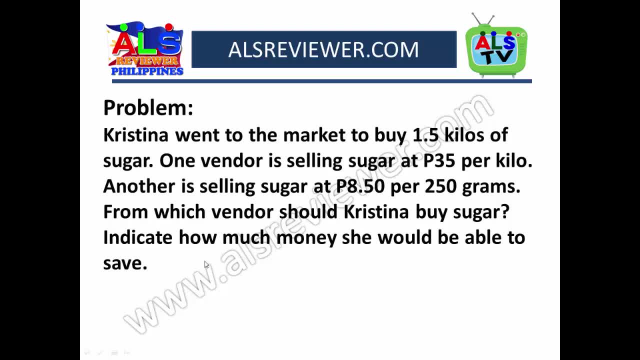 250 grams. from which vendor should Christina buy sugar? indicate how much money she would be able to save? ayan, yung gusto niya makasave saan ba dito? hindi naman parehas ang problema, kasi dito sa presentation 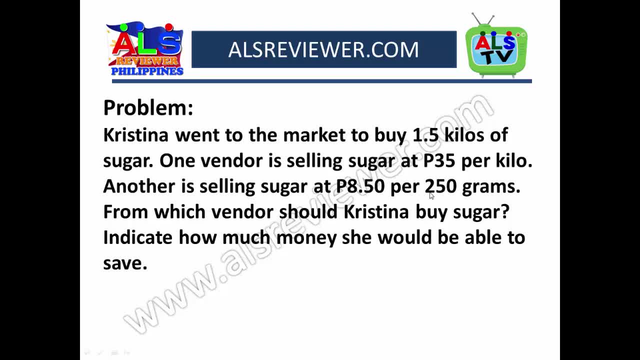 ng problem hindi parehas. yung ibinigay na units, 250 grams yung isa, tapos yung isa naman ay per kilo 35,, yung 250 grams 8.50,. saan ba ako makakatipid dito? yun yung tanong. 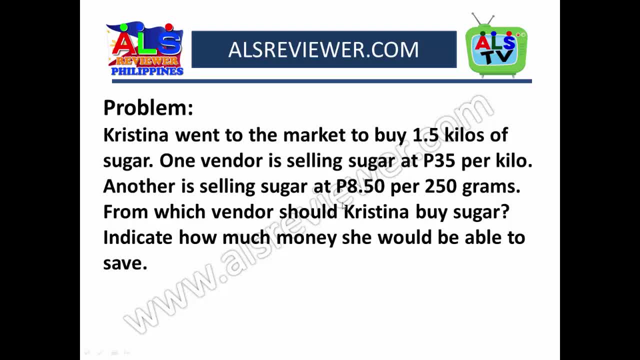 at kung makakatipid ako. magkano so dapat magdesign ngayon, si Christina, kasi maliit lang na bagay yung tinitingnan natin dito. maaring sabi ninyo maliit lang. 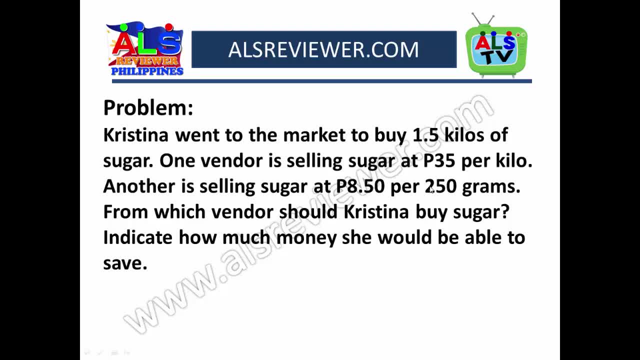 na bagay. pero kung ang pinag-uusapan natin dito alimbawa negosyante ka at gusto mong bumili ngayon ng sako-sakong bigas? ayun kanino ka dapat bumili. 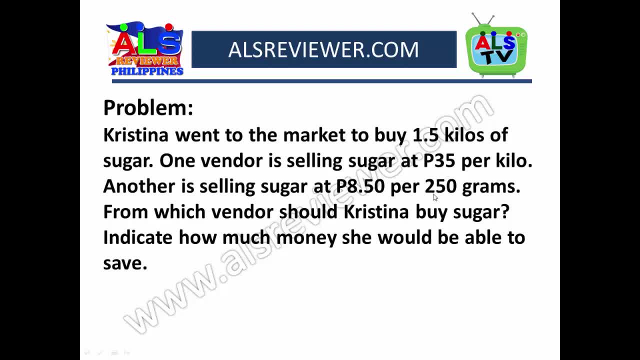 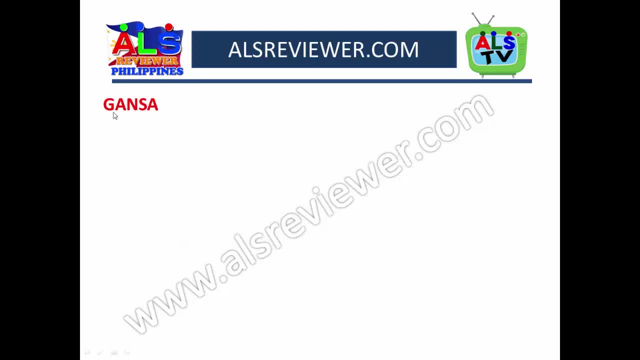 dito sa isa na nagbebenta ng 35 per kilo, or dito sa 8.50 per 250 grams. okay, tingnan natin kung paano natin ito gagawin. so using our acronym GANSA. 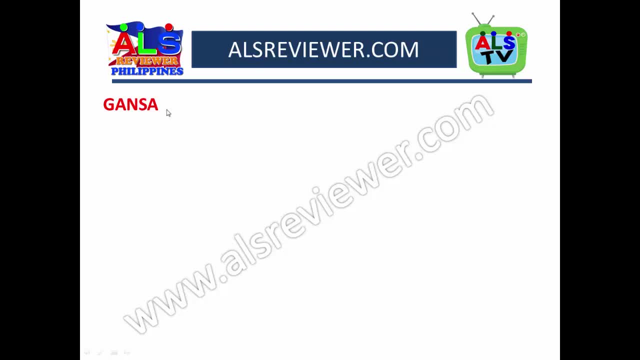 G-A-N-S-A: five steps in solving problem. okay, G given vendor 1 sells 1 kilogram sugar at 35 per kilogram. okay, ito yung given number 1, given number 2: vendor 2 sells 250 grams of sugar. 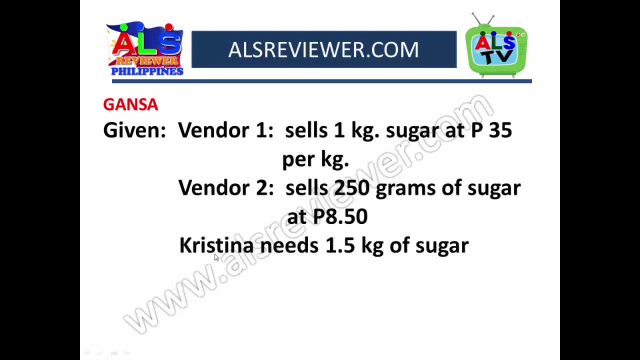 at 8.50 pesos. ngayon naman si Christina kailangan niya ng 1.5 kilogram of sugar. ito yung mga given information. okay, ngayon ang conversion: alam natin 1 kilogram. 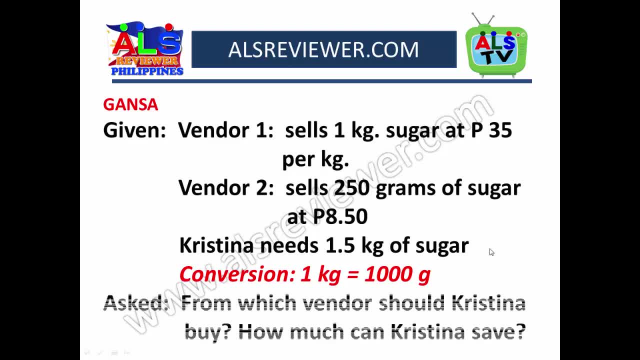 is equal to 1,000 grams. okay, ano ang tinatanong. what is asked? from which vendor should Christina buy at kung saan siya bibili? how much can Christina save, kung tama yung kanyang pinagbilhan sa isang? 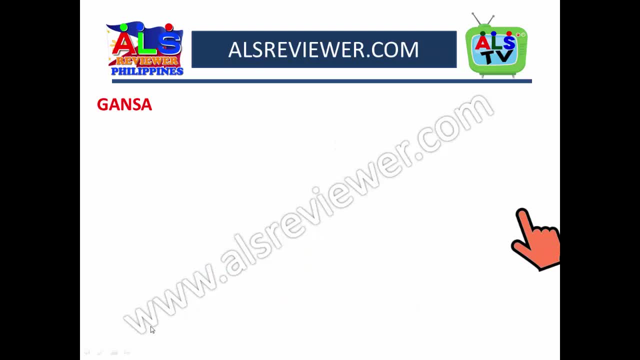 isa't kalahating kilo na kanyang binibili. okay, tingnan natin number sentence natin: let be subscript 1, okay, so gagawin na tayo ng variable para mas madali, kasi pwede naman. 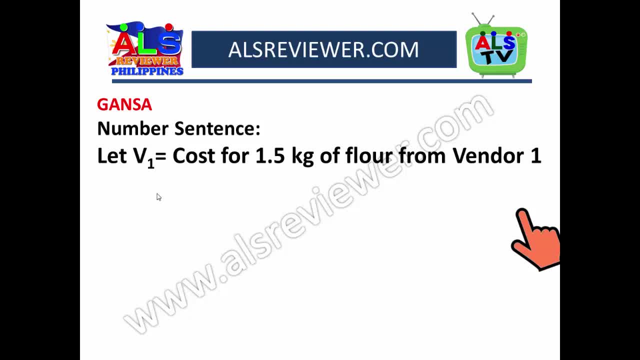 nating sabihin na presyo, ito price 1 is up to you, pero sa algebra kasi pwede nating i-represent yung anon na number with a variable. so V1, vendor 1, yung unang. 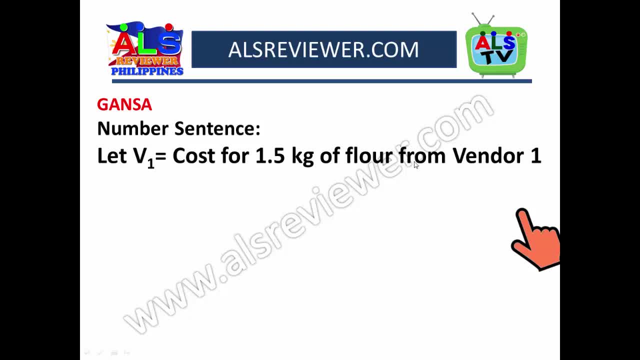 nagtitinda cost for 1.5 kilogram of flour from vendor 1. okay, cost for 1.5 kilogram of flour from vendor 1, so ito yung gagamitin natin. yung V1 let V2 naman. 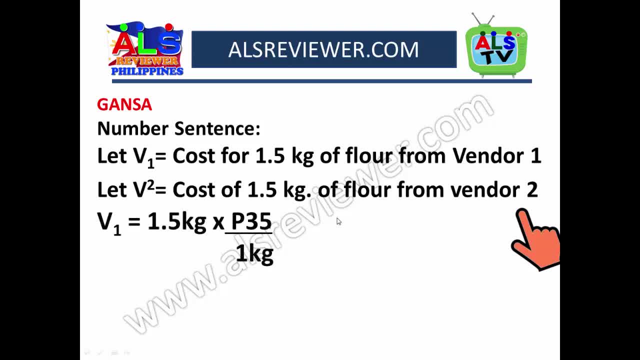 yung cost of 1.5 kilogram of flour from vendor 2 ngayon. eto na ngayon yung ating number sentence. yung V1 equals 1.5 kilogram times 35 pesos over 1 kilogram. 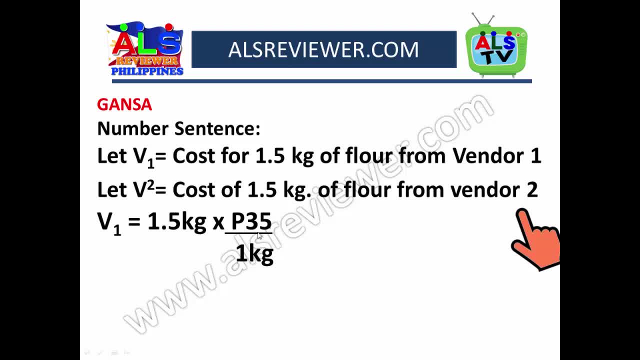 bakit 35 over 1 kilogram? kasi yung 1 kilogram is cost 35 pesos. it means 35 pesos per 1 kilogram and imultiply natin yung 1.5 kilogram dito sa value. ito so magiging 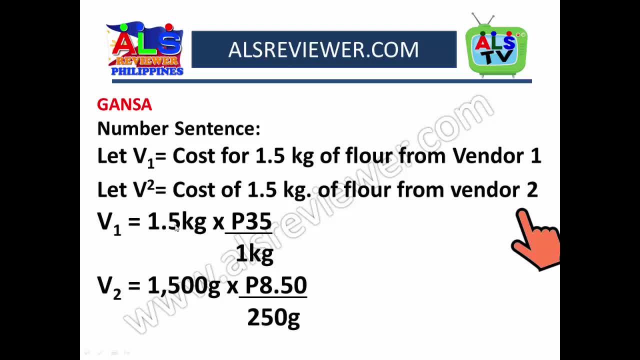 number sentence naman sa pangalawang vendor is: dahil grams, sya 1.5 kilograms converted to grams is 1,500 grams. okay, times 850 per 250 grams. so ito ngayon yung number sentence natin. 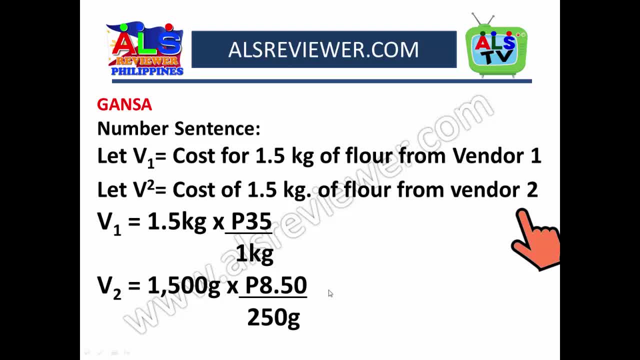 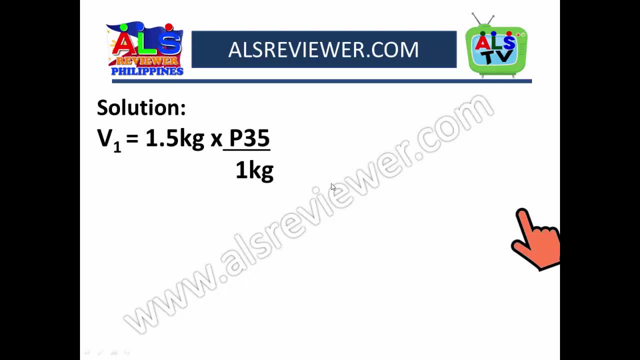 for vendor number 2 or yung price ng vendor number 2, vendor number 1 is equal to 1.5 kilograms times 35 pesos over 1 kilogram. okay, 35 per kilogram ang presyo ng isang kilogram. 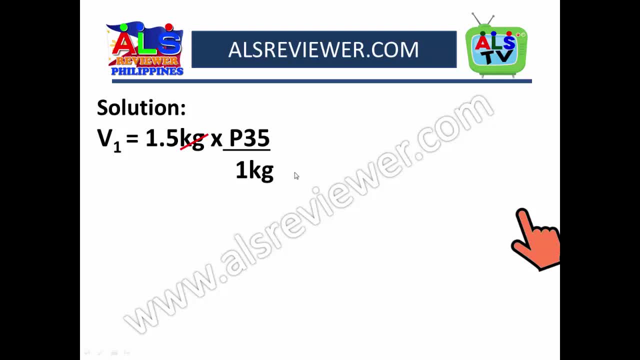 na rice ay 35 pesos. okay, ang sagot nyan pag ika-cancel out natin yung kilogram at saka kilogram, dito ang matitirang unit of measure is pesos, so alam natin na ito yung cost. 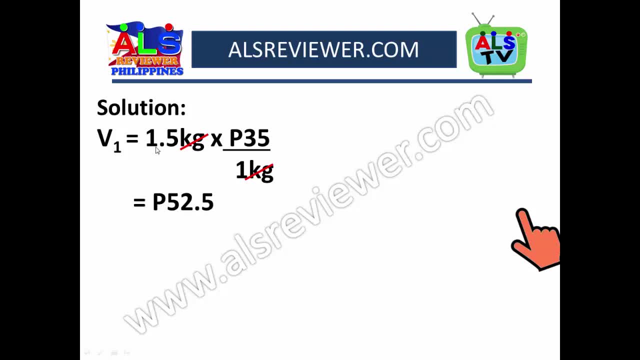 52.5 pesos ang presyo na 1.5 kilograms ng rice dun sa vendor 1. tingnan naman natin ngayon yung vendor 2, dahil ang ginagamit nya is grams dun sa pagbibili. kinonvert lang natin yung 1.5. 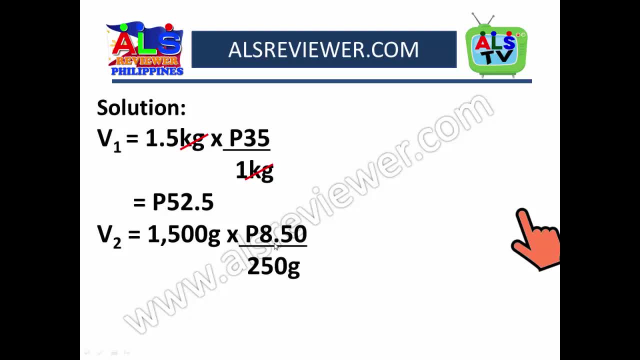 kilograms into grams- 1,500 grams. multiply natin ito ng 850 per 250 grams, so magiging sagot dyan is cancelling out the gram units. okay, ang natitira is yung peso sign, which is pag minultiply natin ito. 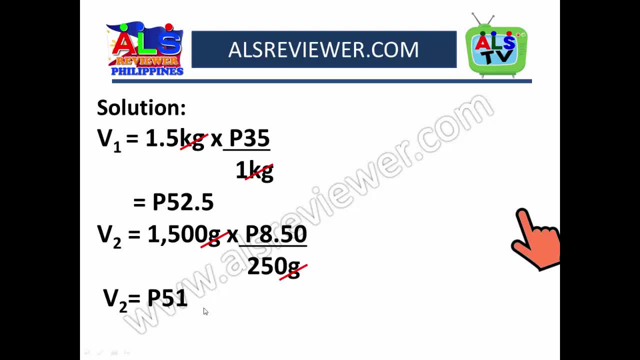 at saka ito didivide natin ng 250, ang magiging sagot is 51 pesos. okay, so ito. ngayon nakita na natin yung value ng vendor 1, which is 52.5 ang cost naman.